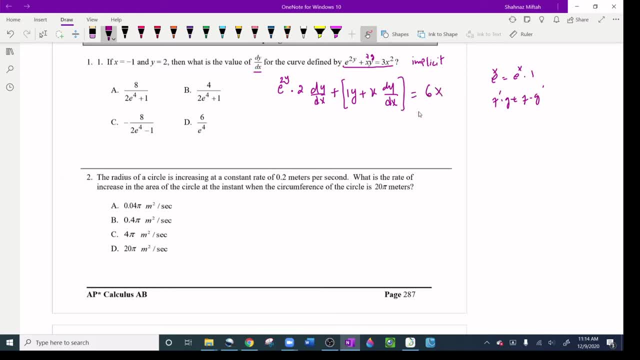 now y function, then 6x. now remove the parentheses and fix this around it. so i got 2e, 2y, dy dx plus y plus x and dy, dy, dx equal 6x. keep all the dy dx is on one side and the other terms on the other side. so 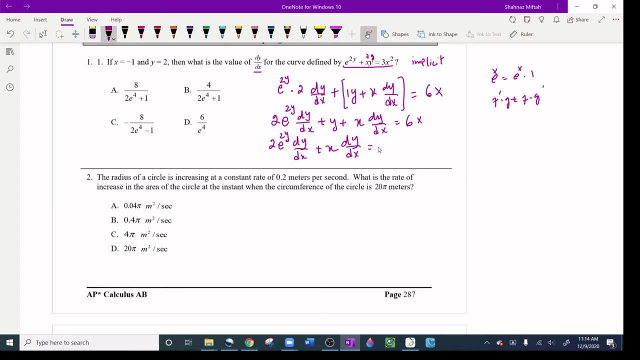 these are dy dx's i'm going to keep on this side, 6x stays and y we subtract, subtract both sides and it's going to come up here now. dy dx is my common factor and we left with 2e 2y plus x and 6x minus y. we divide 2e 2y plus x, both sides and we divide 2e 2y plus x both sides. 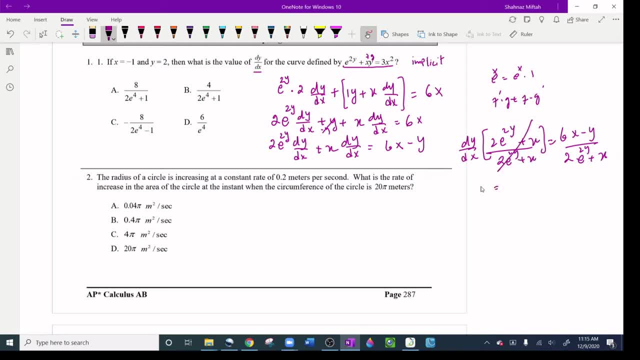 i'm done. now i have to plug in my values. i have a dy dx equal 6 times the x value is negative 1, so it's going to be negative 6 minus y value is 2. i got 2e to the power 4 because y value is 2 2 times 2 is 4 plus our negative 1. x value is negative 1. 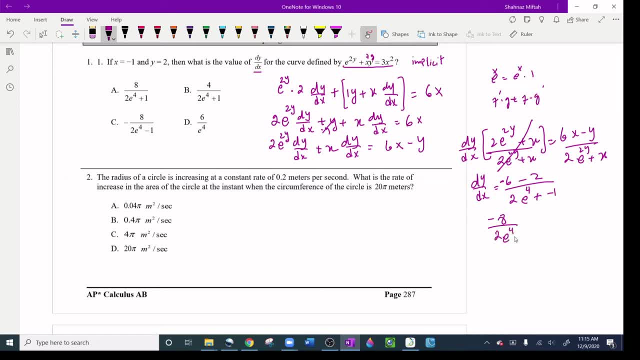 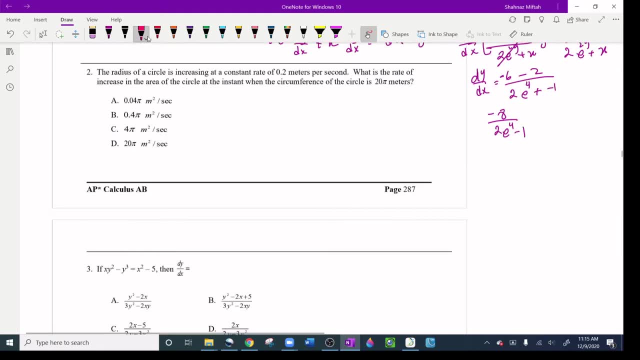 so i got negative 8 over 2e to the power, 4 minus 1. so the answer is c. question number two: the radius of the circle is increasing. that's a related rate question: radius of the circle is increasing at the constant rate. so what is increasing or what is changing at the rate? 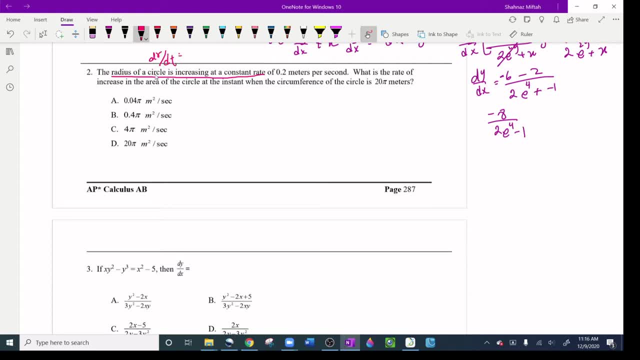 yes, so it means i have a dr dt. whatever is changing at the rate that's a radius, it's increasing. thus 0.2 is the dr dt. what is the rate of the increase in the area of the circle? so area of the circle is increasing, which means d a d t i'm looking for. 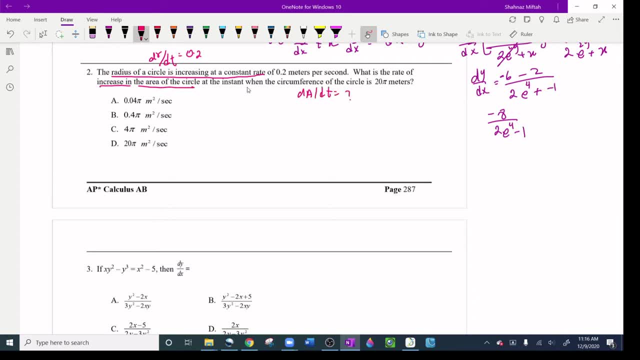 at the instant. instant is also means derivative. when the circumference of the circle is 20, pi circumference is 20. i don't know why they are giving me circumference. we will figure it out, but i'm i start my question, what they are asking me. so, area of the circle, since they are. 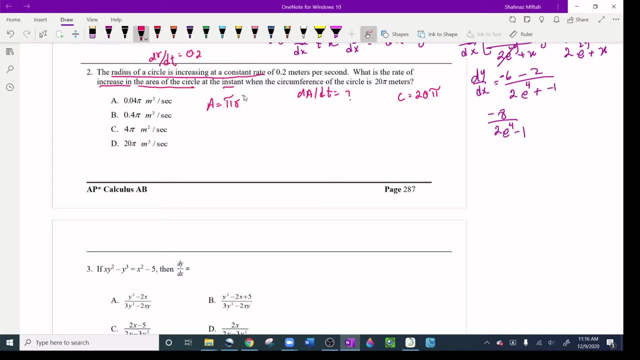 asking d a d t. so area of the circle is pi r square. i'm going to take a derivative d a d t. pi stays 2r dr dt. so r is missing here. do you see? the r is missing. everything else is there. d a d t. 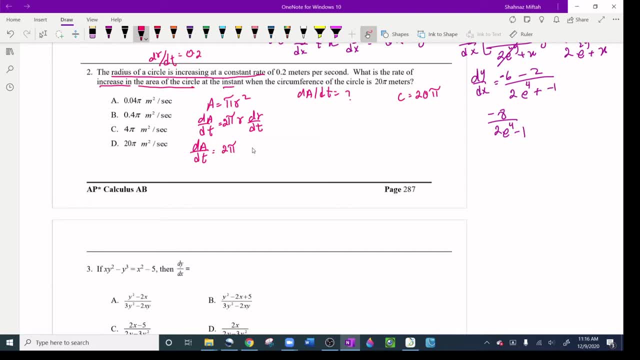 i'm looking for 2 pi r. not there, but dr is 0.2, so i'm missing this r. that's why i have a circumference, so i have to use a circumference formula to get the r. so circumference is 20 pi equal to pi. they are. 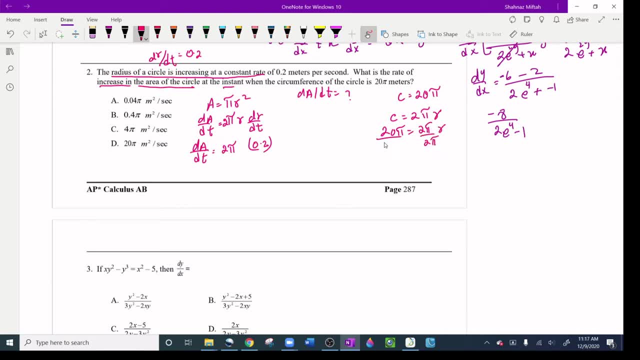 always give me information extra that we need it somewhere, but always start your question, what they are asking you and go from there. so pi pi cancel out. and 2 times 10 is 20, so r is equal 10. so 2 times 10 is 20, pi times 0.2, then it's gonna give me 4, 4 pi. plug this in the calculator, you. 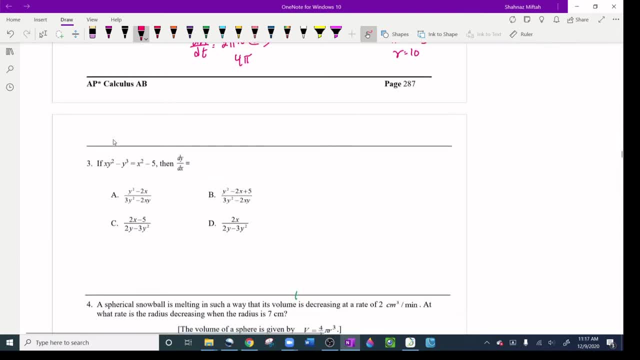 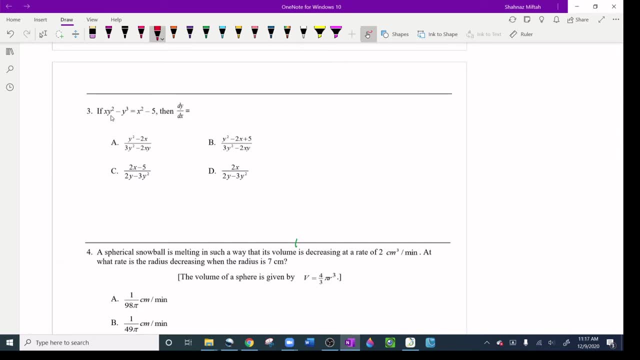 will get that and the answer is c, question number 3. this question is implicit differentiation and you can tell y's and x's are mixed together in x- y. the first one is a product rule. so this is f, that's a g, and the product rule says f prime times g plus f times g prime. so take the. 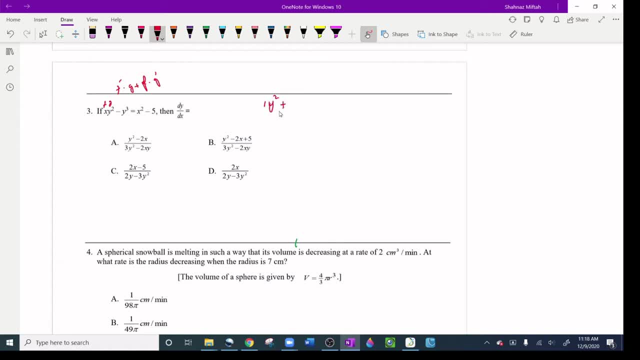 derivative of f, which is 1, keep the y squared plus now i- i put it, i remember i'm putting my rules in the brackets- plus g stays as it is. then we have f stays out as it is x and the y derivative is 2, y, d, y, d, t, d, x. sorry, minus 3. y square d, y, d, x, equal 2 x and the 5 derivative is 0. okay, let's. 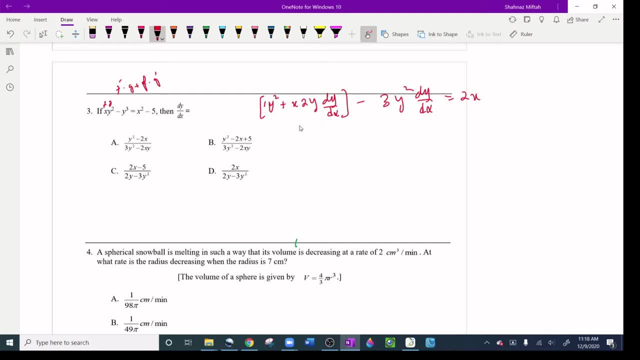 make sure that we keep all the 2, x, y, d, y d. i just move the 2 to the front. d y d x minus 3 y square d y d x. all the d y d x is on one side, the rest of the stuff up here. so i move the y square to this side now. d y d x is my common factor: 2 x, y minus 3 y. 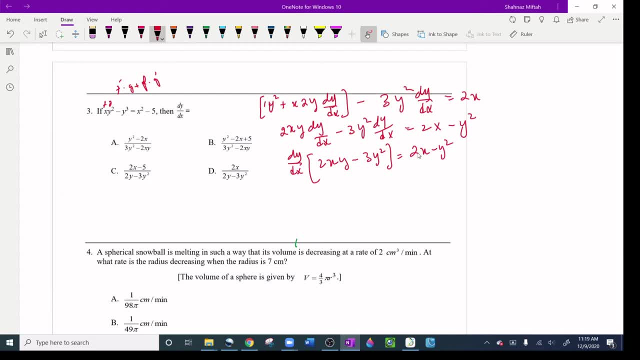 square equal 2 x minus y square, you divide 2 x y minus 3 y square. you divide 2 x y minus 3 y squared. that is my question number three. okay, so let's see what is going on here. so i got this answer, i'm okay, but they always like their answers that in. 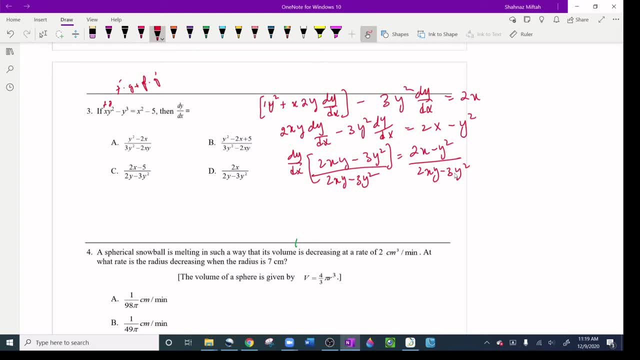 order, like the y square supposed to be in the front. y square supposed to be in the front. so if i do that i'm going to get negative y square, which is not okay. so just multiply everything by negative 1, so it's going to give me positive y square and negative 2, x and it's going to give me positive. 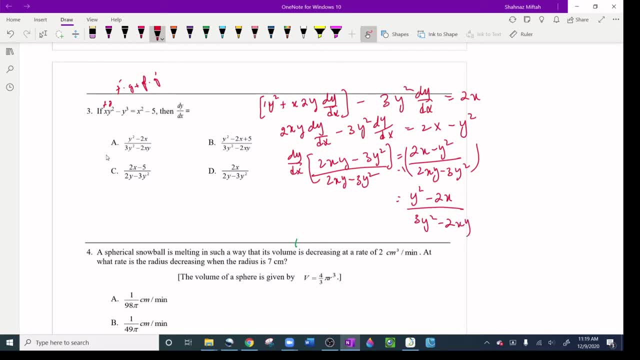 3 y square and negative 2 x y, and you guys can tell the answer is a. and if, if you just stop right there and you check, you're gonna say: okay, y square is positive, negative 2x. so the only difference in this one is the signs, and they switch their places. so it means 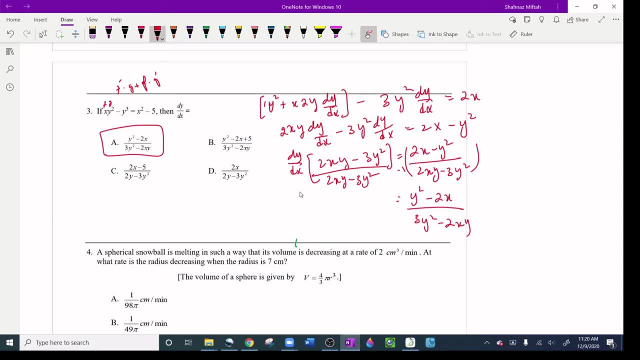 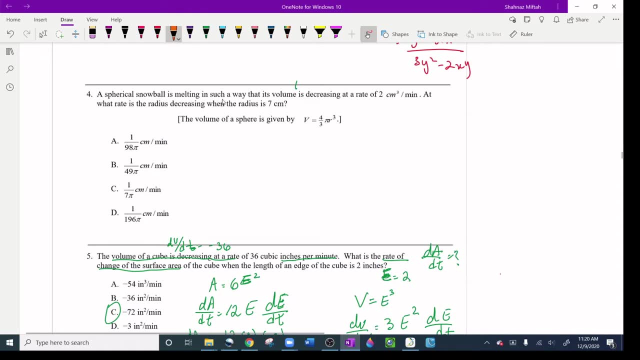 they are multiplying by negative and they are one in order. question number four. question number four is a spherical snowball is melting. melting, which means subtract, in such a way that its volume is decreasing also, you know volume and at the rate. so volume means dv, dt is increasing, decreasing means it's changing. 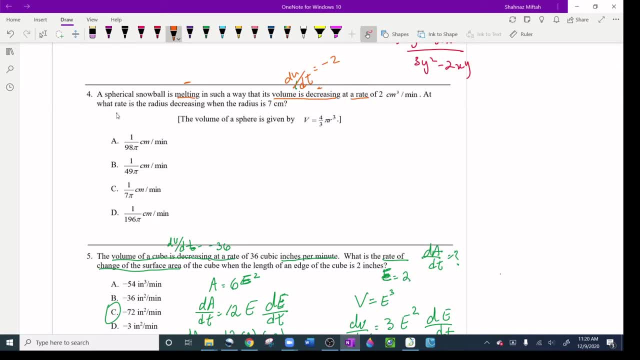 and it's decreasing. then i have negative two. at what rate is the radius decreasing? so dr, dt is missing. whatever is changing is going to be something dt. what is that something changing? or the word rate, or the decrease or the increase? that means changing. radius is equal seven, so volume. 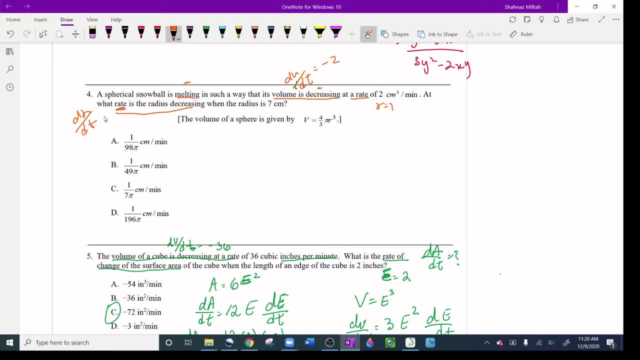 formula of the sphere is this and the question is asking dr, dt. so the formula is four third pi or cube, and i'm going to take a derivative dv. dt equal four third pi stays three r square d or dt. that one is kind of simple. dv dt is 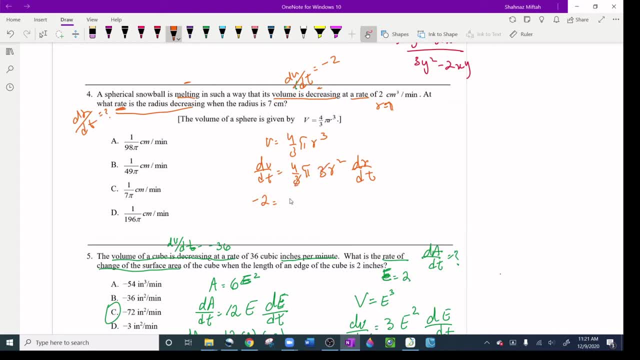 given negative two, three and three cancel out. so, um, i got four pi. r r was seven, so forty-nine, so forty-nine d and d r dt, so forty-nine times uh, four, forty-nine times four, 49 times four is going to give me 196.. so i got 196 pi. 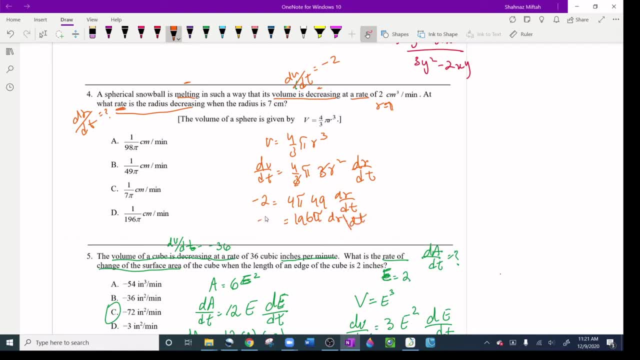 d or dt equal negative 2.. so divide negative 2 by 196, 96 pi equal dr dt. it's going to give me 1 over 98. so my answer is negative 1 over 98 pi. and that's my answer for dr dt. now you will be thinking: why do i have a negative sign here, when 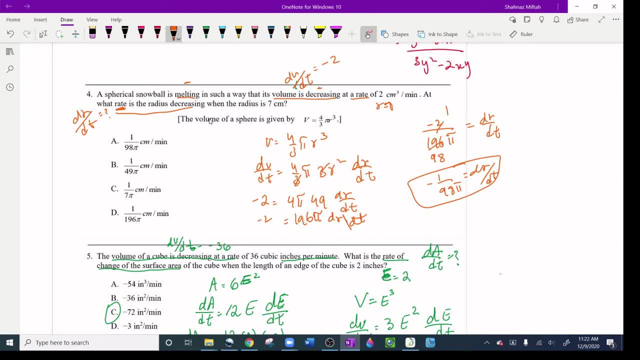 they don't have a negative, since they use the word decreasing, they are already telling me the rate of the radius is decreasing. so when they use the word decreasing, i don't have to put that um, i don't have to put that negative sign there. so that's the reason. question number five: 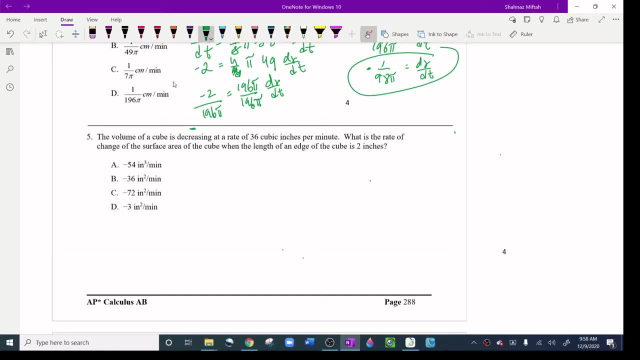 the volume of the cube is decreasing. so what is decreasing volume of the cube when it's changing at the rate? so look for the word rate decreasing, um instance one, when and all of those words. so it says volume of the cube is decreasing at the rate, which means volume is. 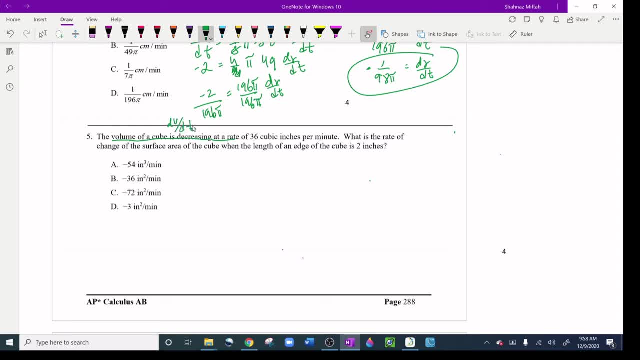 changing, then we should have a dv dt there and it's decreasing, then it's supposed to be negative 36. what is the rate of change of surface area? rate of change of surface area d a, d, t, which is missing, when the length of the edge of the cube is two inches. so edge is two inches. i'm just going. 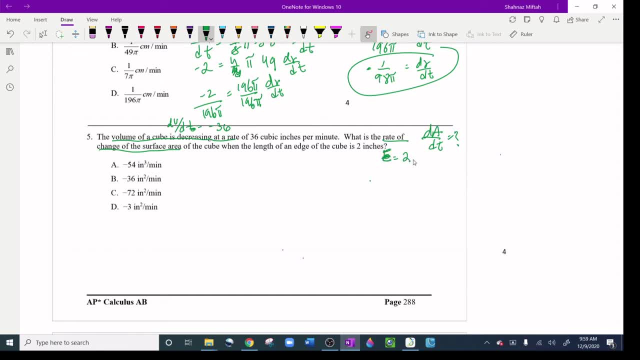 to write e, or maybe just a capital e. this means edge. edge is two. now the formula that i'm going to use, since they are giving me volume and they are giving me area, but i'm going to start what they are asking me first. it's d a d t. so what is the area of the cube? area of the cube is six sides. 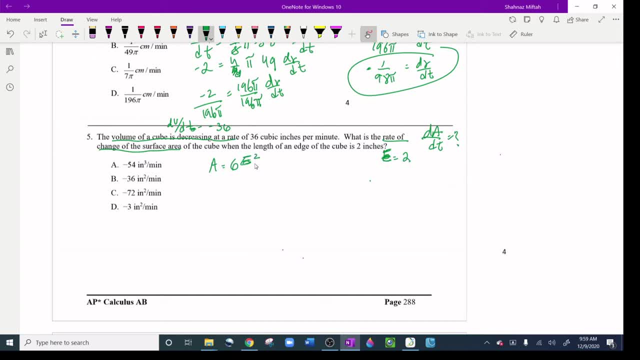 and it's going to be e square, side is e. i'm just going to say side is e, like an edge. so take a derivative of this. it's going to give me d a d t. six times two is twelve e, d e d t, since we have to have a e because the edge is two. and also d e d t is gonna be there because 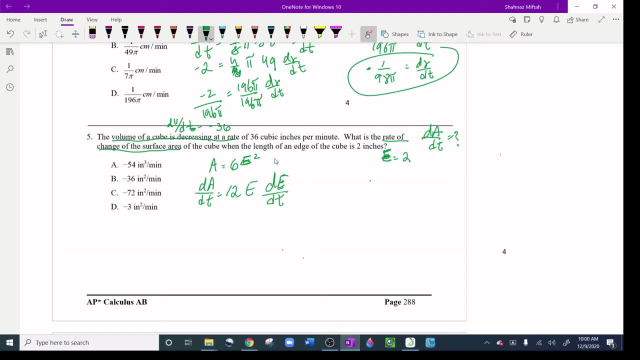 this side the surface area is changing, which means the surface area is changing. then of course, the sides are also changing. that's why the surface area is changing. so d e d t is there, but the problem is we don't have a d e d t, so that's why they are giving me d v, which means i, they want me. 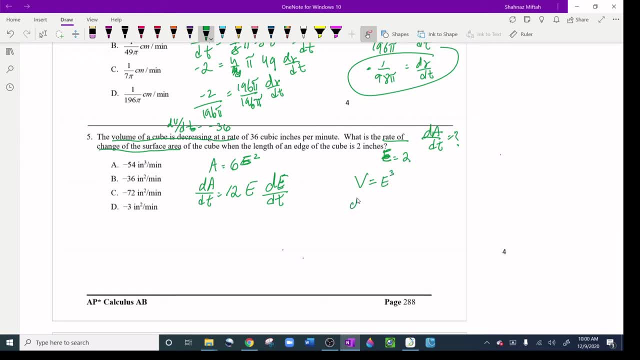 to use a volume formula which is e cube. so let's do the d v d t and use a volume formula. d v d t is given and i will get the d e d t. so 3 e square d e d t. d v d t is negative 36, 3 edge is 2 squared. 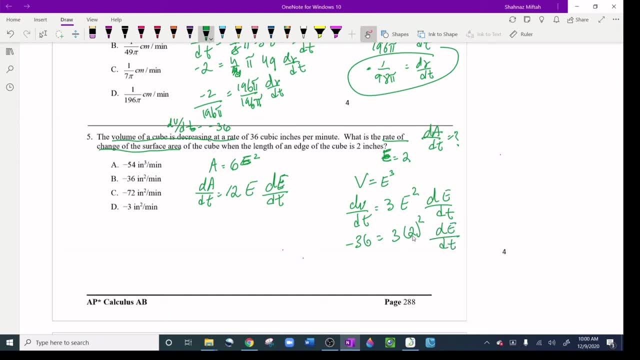 and d e d t. is that what missing? so that's 4. 4 times 3 is 12, negative 36. divide by 12, then it's going to give me d e d t um 12 times 3 is 36. so d e d t is negative 3, so 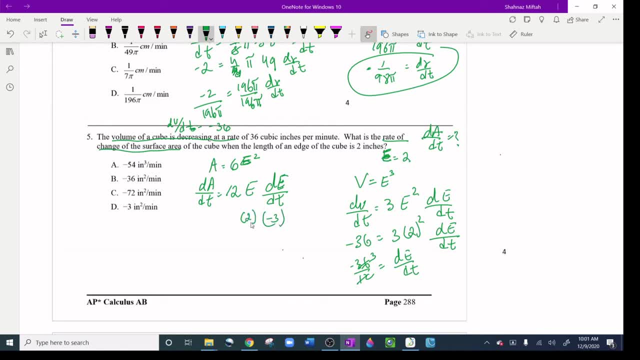 let's put the negative 3 here. the edge was 2 and that's a 12 and d e d t that i'm looking for actually 12 times 2 is 24, 24 times uh. 3, 24 times 3 is uh. 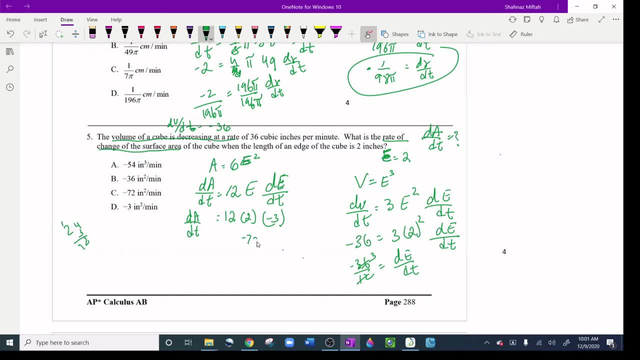 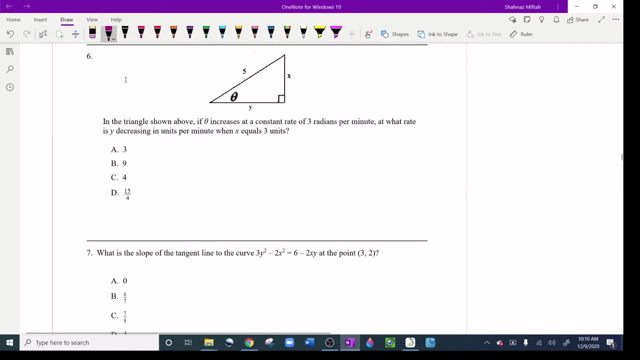 12 and 7 72, so it's going to be negative 72. d a, d, t is negative 72 and since i'm talking about the surface area, the units are square inches square per minute, because that's what it is- inches per minute. so negative 72. the answer is c question, question number six in the triangle above. 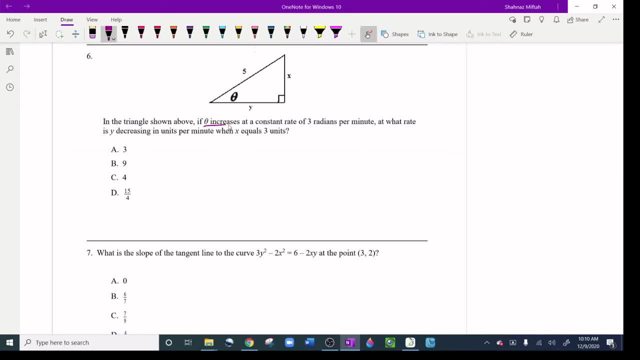 shown above, if theta increases at the constant rate of three radians per minute. so what is increasing or what is changing? and where is the word rate used for? it's used for d, theta, d t, like whenever something is changing. that's where d something, d t is gonna go, at what rate? the y is decreasing, which means 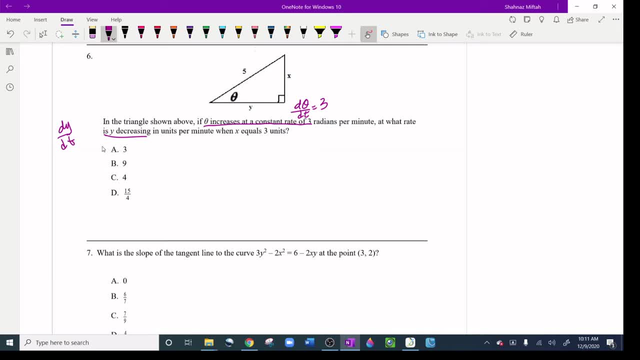 d y d t, they use the word rate decreasing, that's d y d t, and i'm not looking for that when x is equal three, so we use the word rate, and i'm not looking for that when x is equal three. so we use sokotoa here, because they are talking about d theta d t and d y d t. so um, if i use cosine, it's. 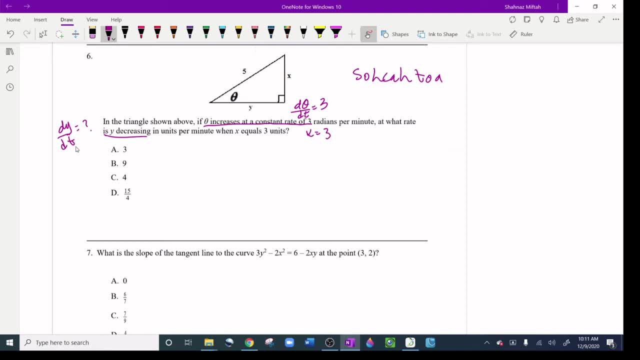 going to be adjacent because i have to have this y, since i'm looking for d, y, d, t now i have to have a y in the trig function, so adjacent or hypotenuse would work. so i have cosine theta, adjacent y over five. i'm going to rewrite this like one-fifth um cosine theta. 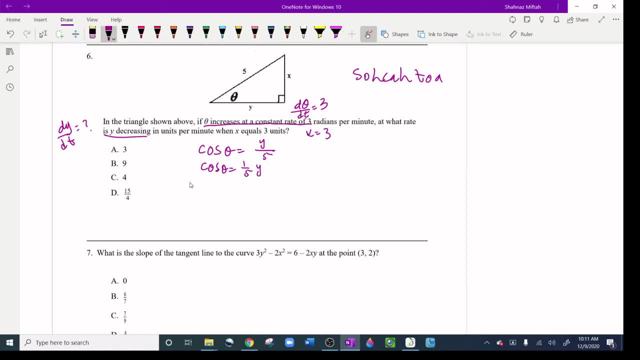 one-fifth, y like that and then take a derivative, so cosine derivative is negative sign. keep the inside, that's outside, that's inside. keep the inside as it is and the inside derivative is one and we're going to keep the d theta, d t with it. one-fifth, and y derivative is one and d y d t. 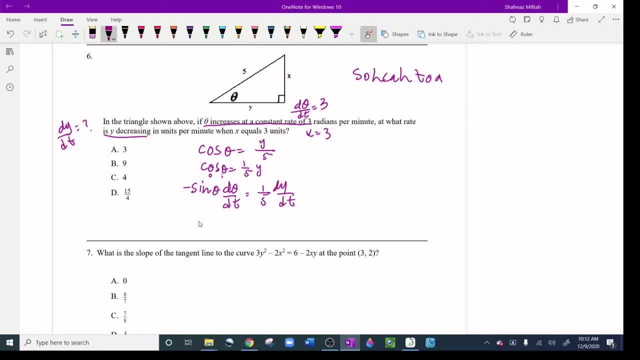 since i'm taking a derivative of y and y is changing, theta is also changing because d theta d t is given in the question. so now, uh, what is sine? what do i plug in for sine theta d t? we know it's a three. so what is or do i plug in for sine theta? sine means opposite, and 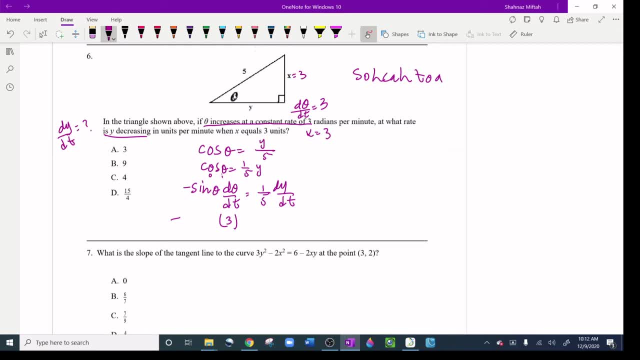 hypotenuse, so opposite is three. hypotenuse is five, so three over five. uh, three over five is sine opposite and hypotenuse, yes, equal one-fifth d y d t. now, three times three is nine, so i got negative nine over five. and uh, i'm timing five equal d y d t. i moved this five. i multiply five both sides, or you can: 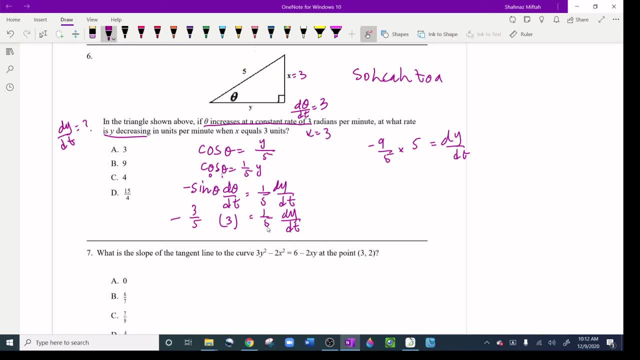 do the division divide one-fifth both sides and you do reciprocal, it will be the same thing. five, five, cancel out. and my answer is nine. since they use the word decreasing already, i don't have to put that negative. so i got d y d t. you're going to say d y d t is equal nine, and uh, it's uh. 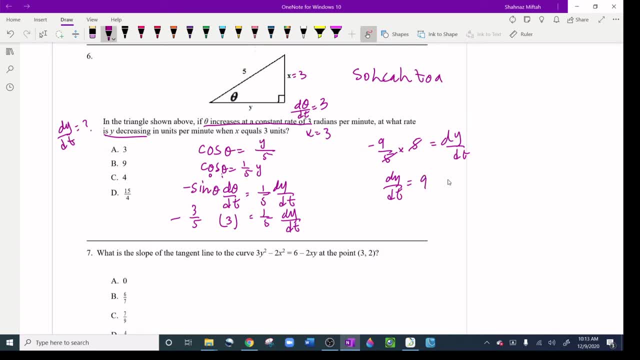 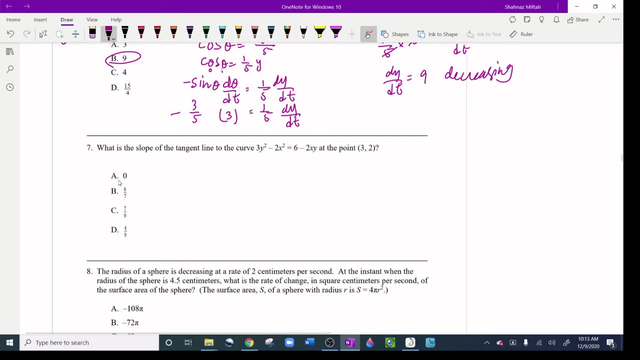 decreasing. so when you use the word decreasing you're going to say d y, d, t is equal nine, so decreasing don't put the negative sign. so the answer is b. question number seven: what is the slope of the tangent line to the curve? uh, three y square minus x square equals six minus two x y. at the 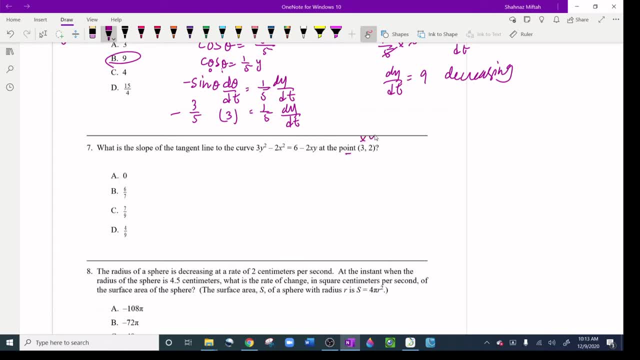 point three and two. point means x and y values and since they said tangent, it's a derivative and the slope? we are only looking for the slope, so i have to plug in these values once i take a derivative. so let's take a data and this is implicit function. this is implicit, so i have to. 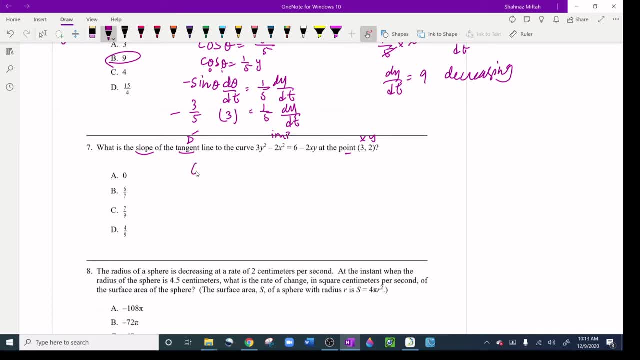 do the d y, d x. take the derivative and the tangent line to the slope. so i have to plug in the derivative of three y square, which is six y, uh, and taking derivative of y means d y, d x minus. take the derivative of x and we don't put d x, d x, um. this is a product rule minus two. i'm going to keep it. 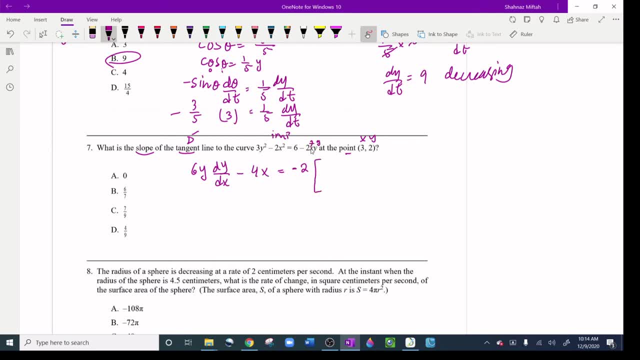 and i make product rule: that's f, that's the g f derivative is one. keep the g plus f stays and g derivative is one. and we're going to keep d y d x there. now let's fix around the stuff: d y d x minus f. and we're going to keep d y d x there. now let's fix around the stuff: d y d x minus f. 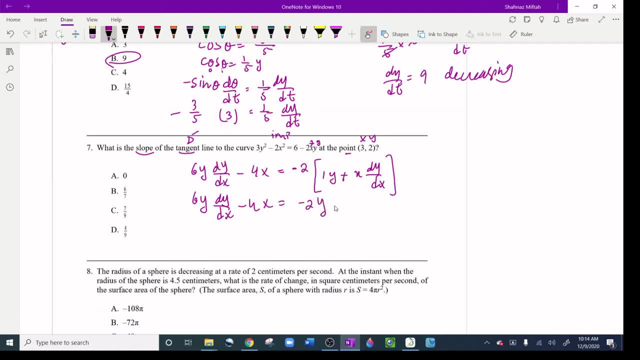 minus four x equal negative two, y minus two x, d y d x. now, uh, plug in the numbers. two is a y value, so six times two is going to give me and d y d x i'm looking for actually. uh, minus four times three, negative. two times two minus two times three and again d y d x. so six times two is twelve. 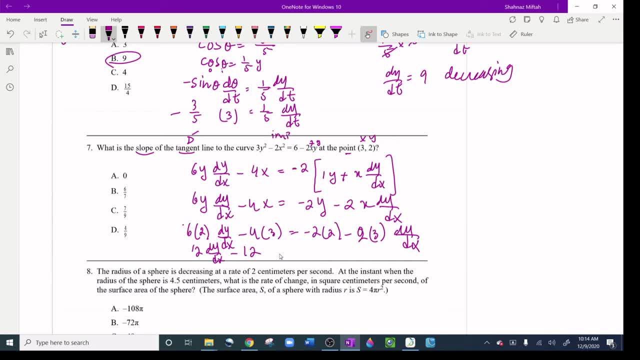 d y d x. and again d y d x minus four times two is twelve. and again d y d x minus four times three: dy dx. negative 12. negative 4 minus 6. dy dx. combine all the like terms. so i'm going to keep the dy dx. 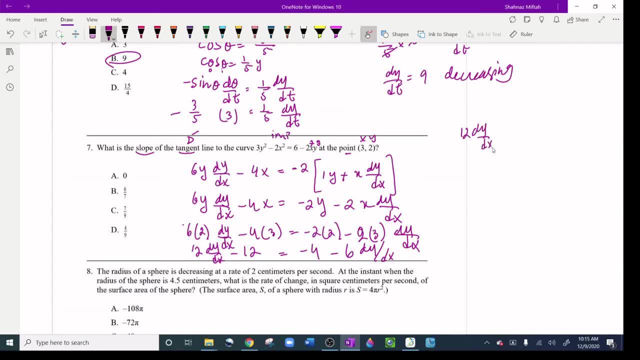 on one side. so i got 12 dy dx and plus 6 dy dx because i moved that negative 6 to the other side of equal and change the signs dy, dx, equal, then 12. i moved to the other side of equal and it's turned positive and minus 4 stays 12. subtract 4, 12, 11, 10, 9, 8, so it's going to give me 8 and 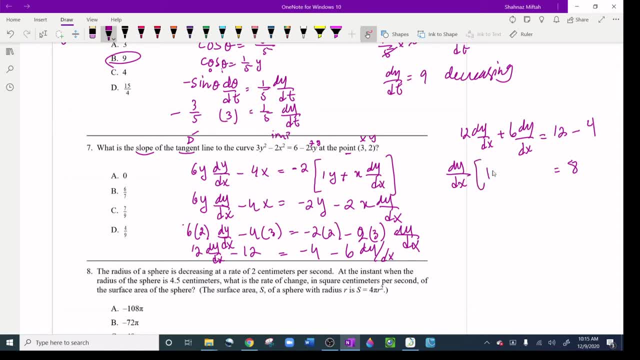 dy, dx is my common factor, so i got 12 plus 6. inside 6, 7, 8, i got 18 technically, so divide 18 both sides. this is also 18 actually, okay, so i'm just going to erase it in 18, uh, 8 over 18 and we 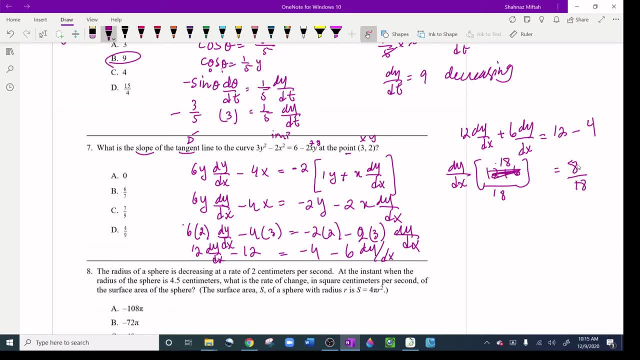 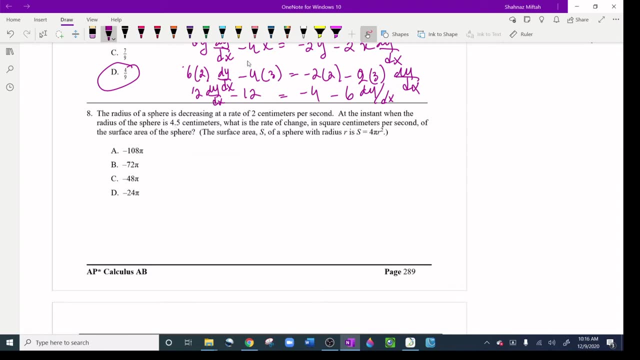 simplify this: um um, two times four and two times nine, so four over nine and the slope is four over nine. question number eight: the radius of the sphere is in decreasing, so let's do that radius. radius of the sphere is decreasing at the rate of two sphere radius, so dr dt is equal negative. 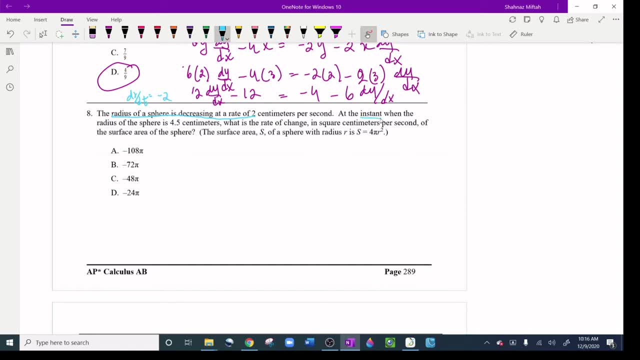 two, because it's decreasing at the instant. instant is also something like instantaneous rate of change. that's a derivative. so that's a derivative d something when the radius of the sphere is 4.5 at the instance. instant when the radius is 4.5. so that's 4.5 radius. we're going to plug it in when, after we 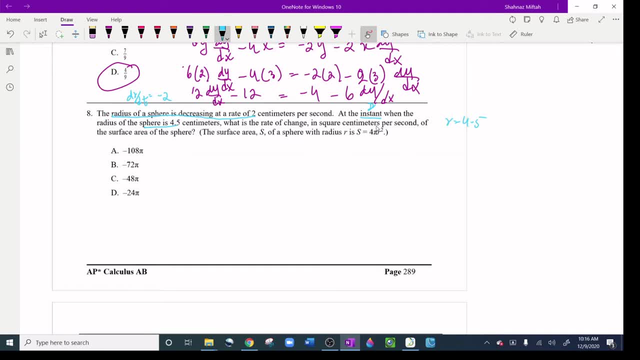 take a derivative. what is the rate of change in square centimeters per second of the surface area of the sphere? so, rate of change of the surface area, so d a, d, t i'm looking for surface area of the sphere is 4 pi r square. so let's take a derivative of this and see, and you. 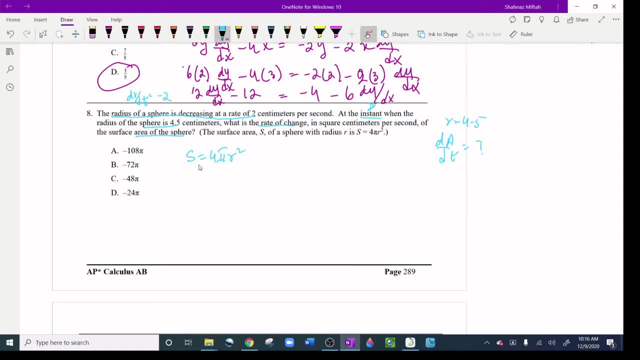 know the d a d t. i don't have a d a d t in here because if i take a derivative, uh, surface area, i'm sorry. so it's going to be a. i just put the s, that's surface area, a. so i'm going to go d a d t. 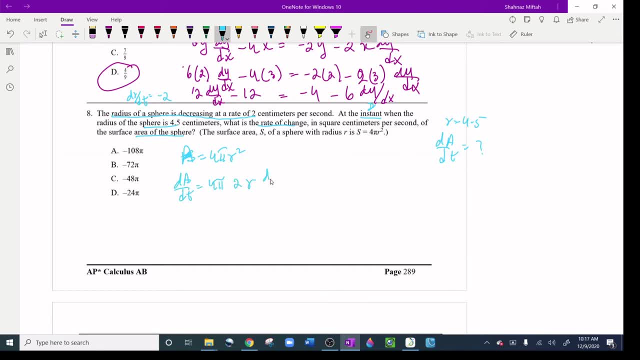 4 pi stays. that's a coefficient 2r in dr dt. plug in everything. 4 pi times 2, radius is 4.5 and dr dt is negative 2.. so this is going to give me um, let's try that. pi is going to stay as a pi, so 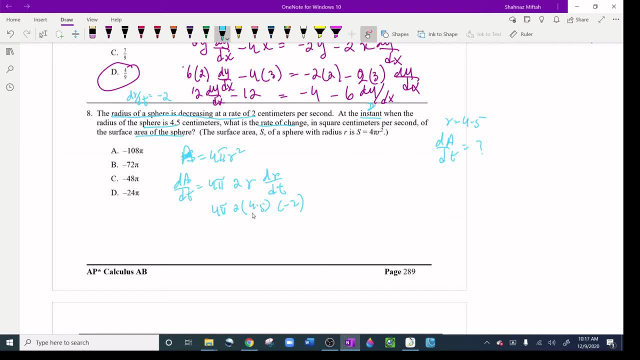 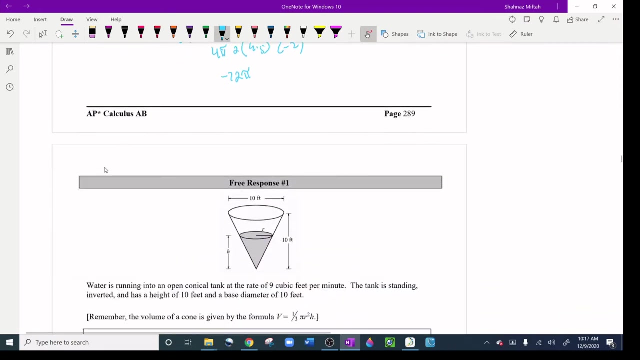 2 times 4.5 times negative. 2 is negative. 18 times 4 is going to give me negative 72. so my answer is negative 72, pi, which is uh b. so these are all multiple choice questions. now here we go with the free response. 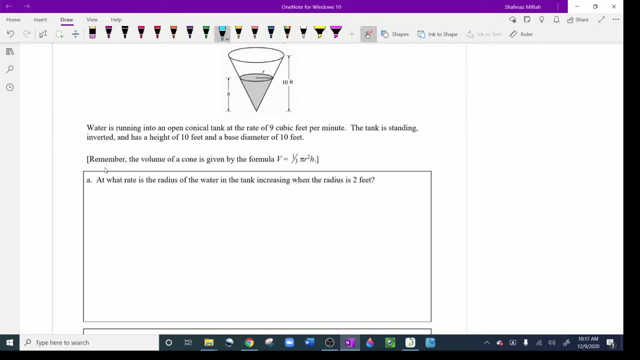 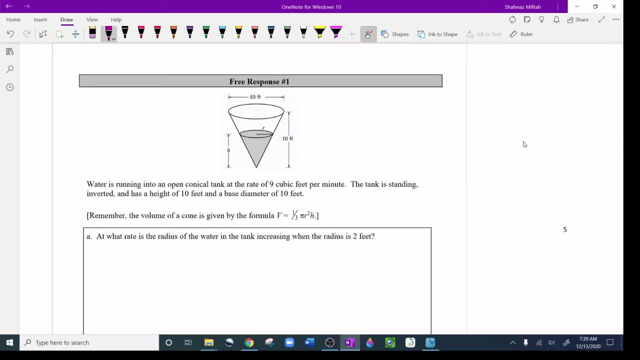 questions of test number four: free response: uh, part a. in this free response, all you have to do is read the question first carefully. water is running into an open conical at the rate of nine cubic feet per minute. since it's cubic and uh, it's also said rate. 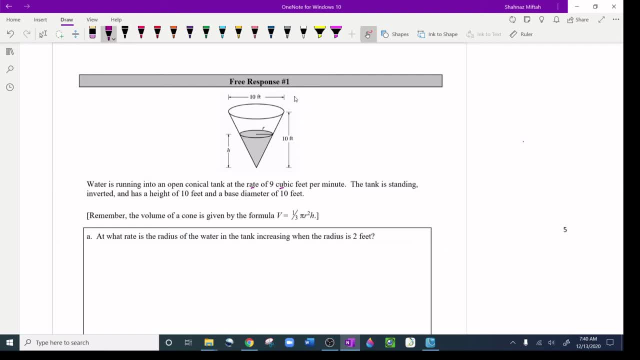 running into the open conical, so running water is running into it at the rate rate means d something, dt anything changes of nine cubic. so it means it's volume, because cubic goes with volume. so dv dt is equal nine. the tank is standing inverted and has a height of 10 feet and a. 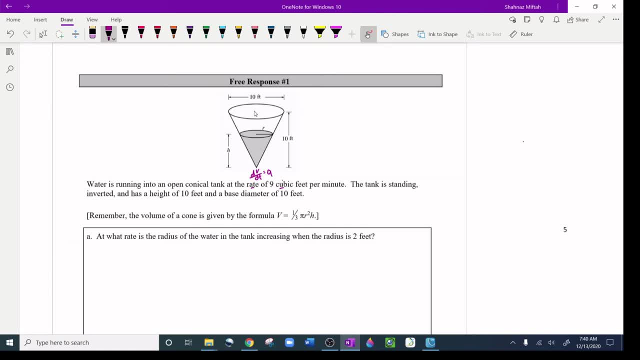 base diameter of um base diameter of 10 feet. so it means the radius of the cone is five and the height of the cone is uh 10.. now this is the water right there. that's this. the exposed surface, uh, is a circle, and that's radius of the water, which we don't know. 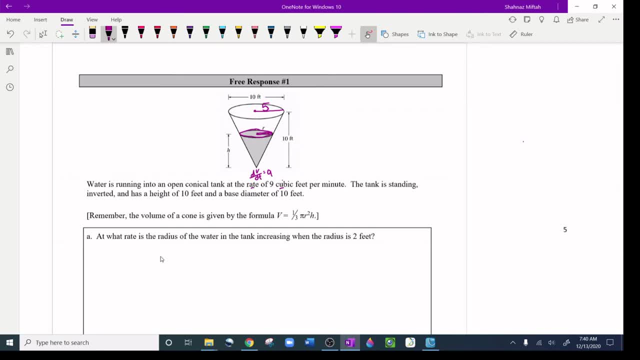 height of the water? we don't know. remember, the volume of the cone is given by the formula this: at what rate? at what rate, which means d, something dt is the radius, which means the rate is the radius, so dr dt of the water in the tank increasing. since radius is increasing it, it means dr dt. still, when the 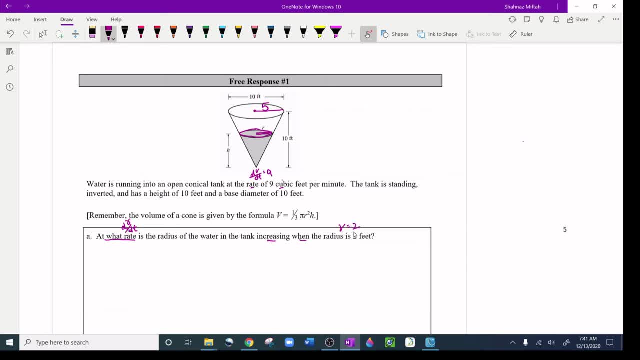 radius is two feet, when, after the derivative. okay, so let's uh put the volume formula, which is one third pi r square h, and i told you guys this before. it's a cone, remember the proportion, don't? uh, don't forget that. keep this in mind. probably we need a proportion, okay, pro portion. so let's see. 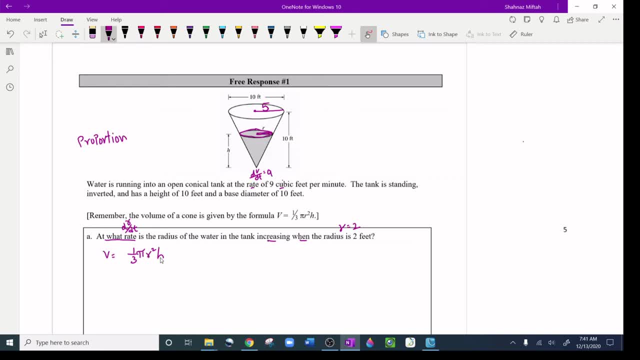 uh, i'm taking a drill in my head. it's gonna r a r square h means it's a product rule and i'm gonna have a dr dt and i'm gonna have dhdt. do i have all that stuff? and if you guys pay attention, i 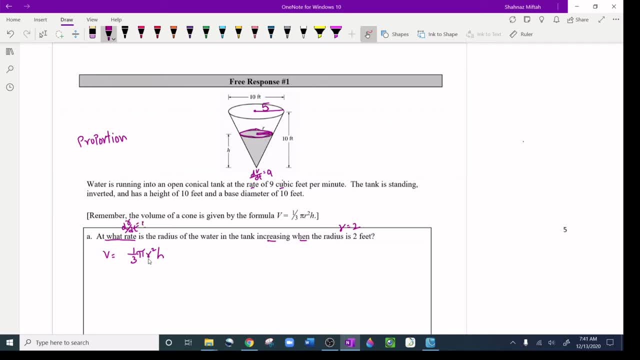 i'm looking for dr dt, so we cannot remove the r, but do we have a? do we have a dhdt? no, and we don't have a height of the water either, because we are talking about rate. is the radius of the water in the tank increasing? so we're talking about the related rate, or this whole thing is? 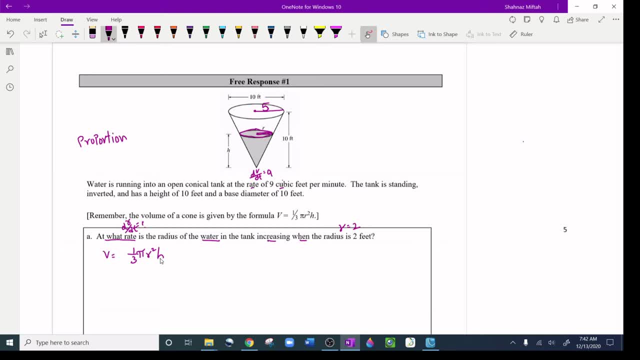 talking about water, so not the cone. so an h is not given for the water and we don't have a dhdt, so it means we have to get rid of this h. so how would we get rid of the h using a proportion so r over h? 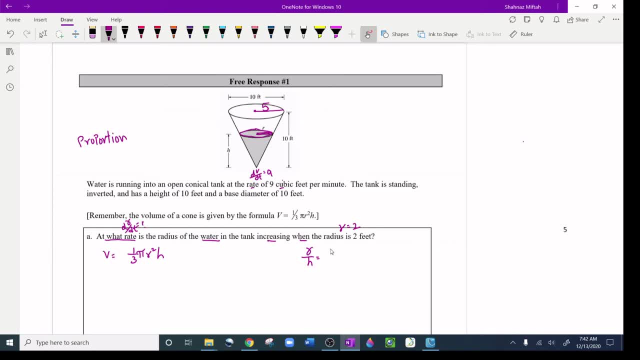 like the radius of the water in the height of the water. now, radius of the cone is five and height of the cone is ten. they have to be exactly the same, like that. so you cross. multiply them. i am getting 10 r equal 5 h, and since i need to get rid of h, 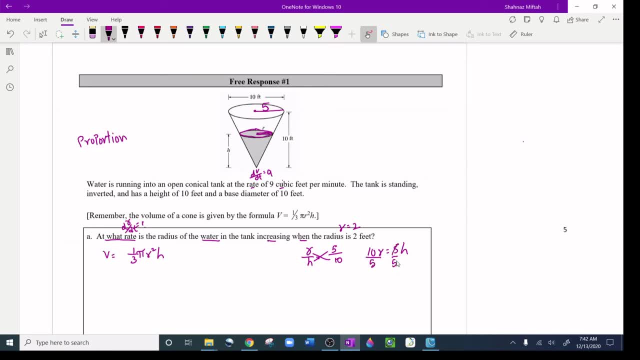 i'm going to make the h by itself and i will replace it with this half two. so i got 2r equal. I'm gonna box it and I'm gonna replace this H before the derivative. because we don't have a DH, DT R square for the H, I'm gonna type in 2 R, so I did that now. 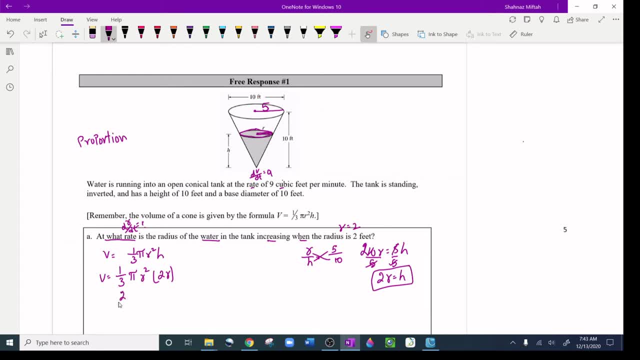 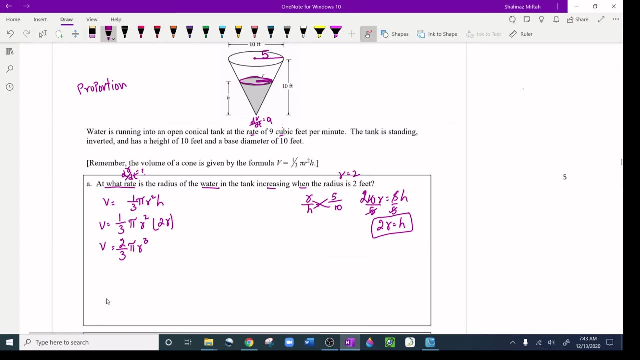 simplify this. I am getting 2, 3rd, 2, 3rd pi, R cubed, R square and R 1 multiplying, so it's gonna go R cubed. now, this is my formula. now I'm gonna take a derivative of it. so let's take a derivative: DVD T equal to third pi. derivative of R cube. 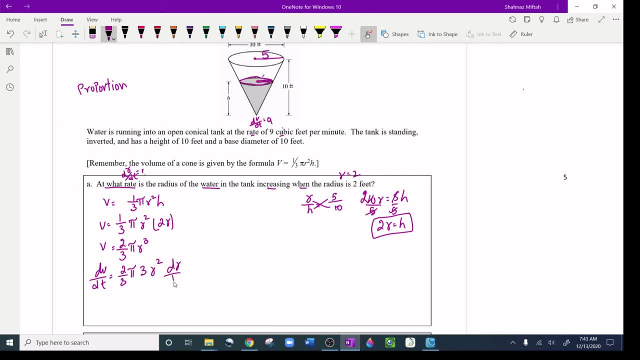 is 3 R square in D or D T. now DVD T is given in the question, which is 9, 3 and 3. cancel out. I'm left with 2 pi. what is R? R was 2 after the derivative, which means 2 squared. 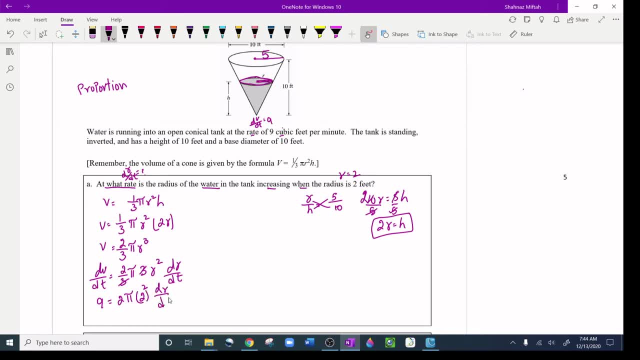 in D R D T. I'm looking for it. you have to do: give them all the things step by step. 4 times 2 is 8 pi, D R D T equal 9. now divide 8 pi both sides and you will get D R D T. should I some? I can simplify this further, so that's my answer. so 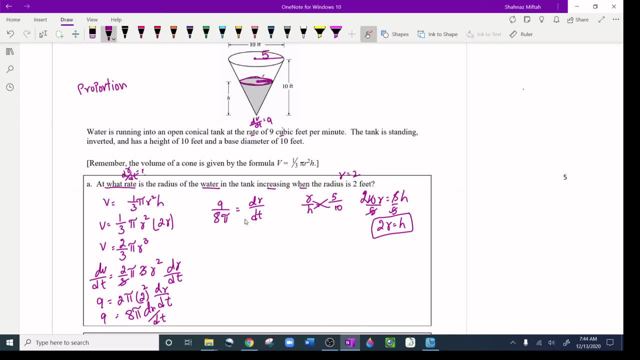 write the units. where are the units here? I have feet per minute and since it's a radius, it's gonna just feet per minutes and radius mean the derivative of the radius, like it's a rate rate. always go with the per feet per minute. and this question, this. 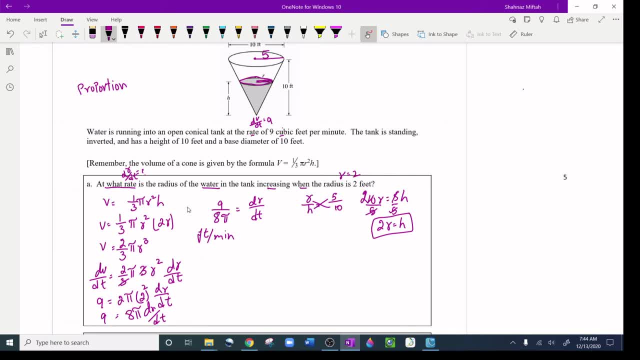 section of the part a is three points. it has three points. one point: how would you replace this H with 2 R, like all of this and replacing it and getting the new for new original formula? that's one point. the derivative is the second point in the answer, is the third point. so you 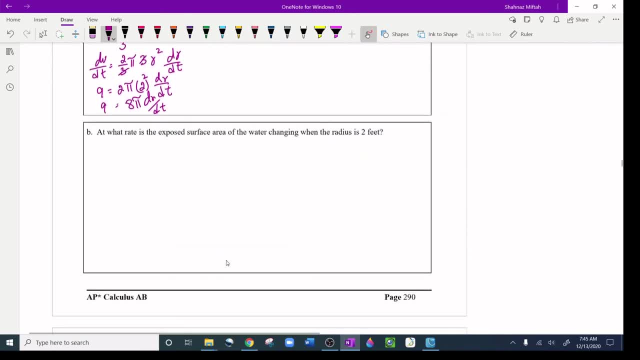 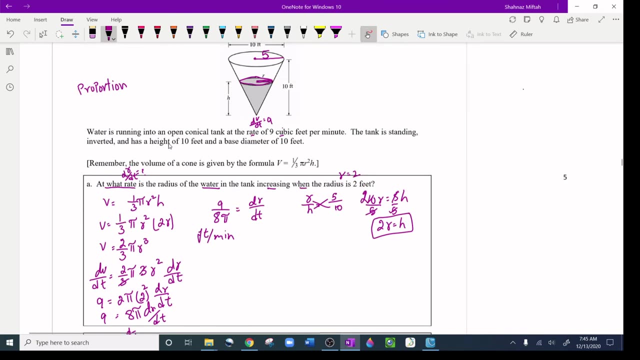 have three points on this pot. a: let's do port B, port B's target, at what rate? at what rate? again, D: something DT is looking for exposed surface area, surface area of the water exposed. and if you are shocked, I just said exposed surface area of the water is a circle that's exposed. this is what we can see when we look at. 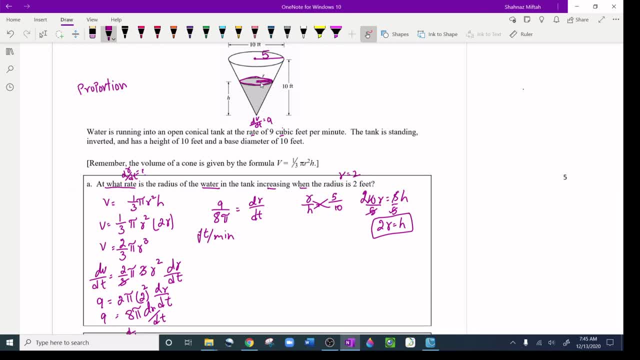 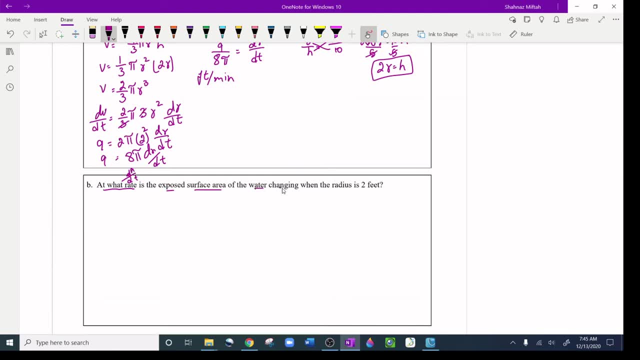 on top of this cone. it's a circle, so exposed area of the water is circle, so surface area of a circle we're talking about. so i'm gonna say d a d t of the water changing again, d a d t when the radius is two. again, area formula of the circle: it's pi r square um. now take a derivative in the head: d a d. 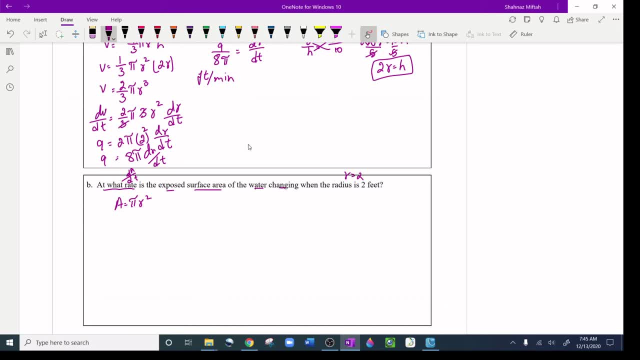 t to pi or d r d t. do we have a d r d t? we got d r d t up there in the question part a, which is nine over eight pi. so we are, we are okay. so i'm gonna take a derivative d a d t equal two pi r d r. 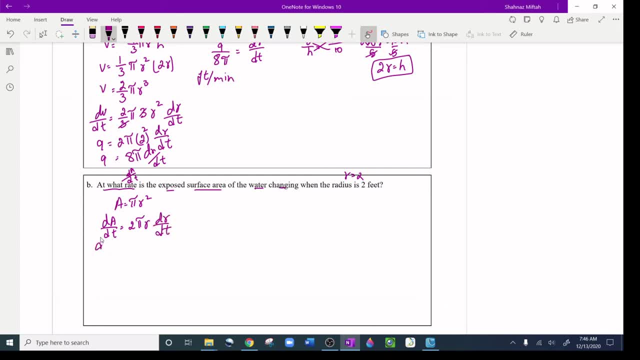 d t, d a d t i'm looking for, so it's gonna stay here. two pi and r is two, and what is d r d t? it was nine over eight pi which we got in the first uh part a, so two times two is four, four pi pi. 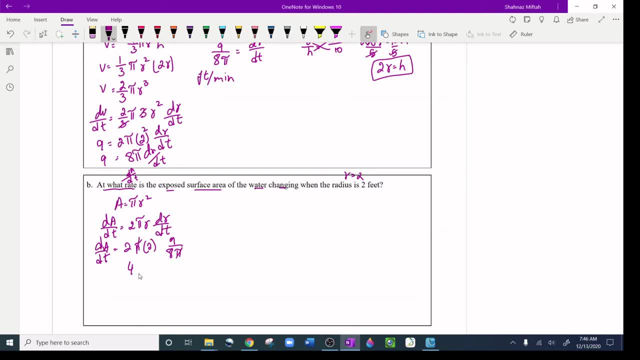 cancel out you and uh a nine over eight. now simplify this further: d a d t, d a d t over 36 over eight. so uh well, 36 over eight. it's gonna give me uh four times two is eight and four times nine, so nine over two. and since i'm talking about area it, 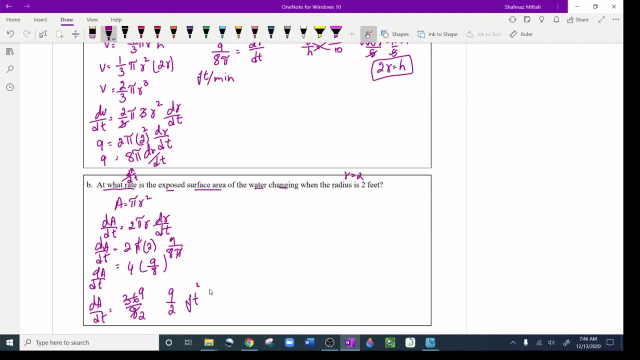 has to be six. so i'm gonna take a derivative of that and i'm gonna take a derivative of that and square so feet square per minute per, because of the derivative d, a, d, t like a rate. this is a rate, so nine or two feet square per minute. so this part b has three uh points: two, one point taking. 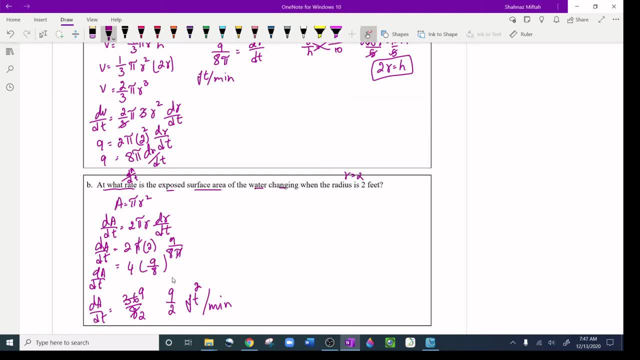 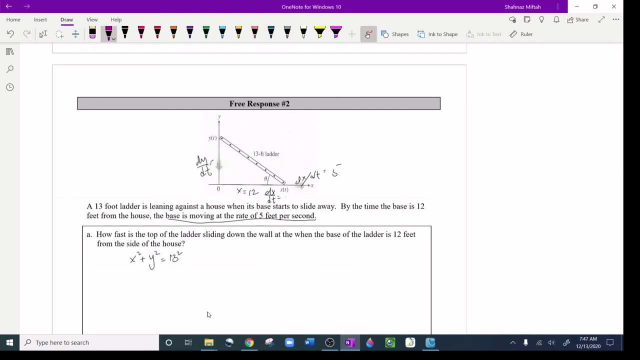 a derivative? second point: how do you plug in, like the value in part a, like you did plug in this nine over eight? that second point in the third point is for the answer. let's go for the next question. this is a response number two, free response, and this all the. 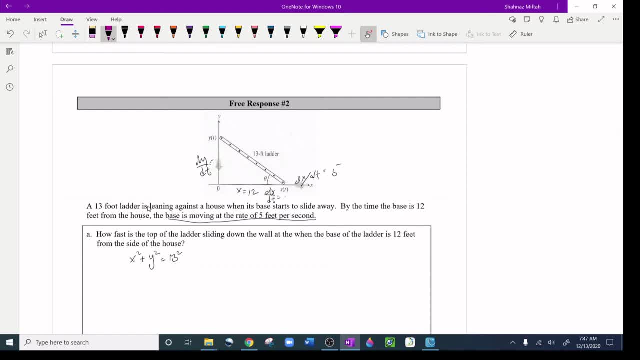 information is given right there. they are talking about a 13 feet foot ladder is leaning against a house. this is 13. when its base starts to slide away, the base slides away. by the time the base is 12 feet from the house. like this is axe and it's tall. the base is moving at the rate of five. 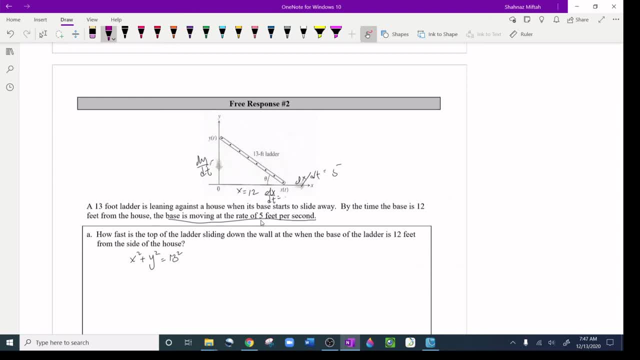 feet per second. so the X DT is your five. that's what the that this is moving. now, first part: how fast is the top of the ladder of sliding down? this is top of the ladder. it's sliding down. how fast means? I'm talking about rate again. so technically I'm talking about dy DT is missing. 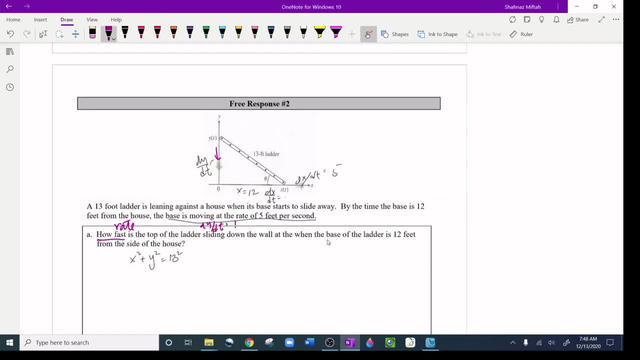 so dy DT I'm looking for. so right down here dy DT question mark when the base of the ladder is 12 feet from the side of the house. so this X is going to be at 12. and they said: figure it out the rest of the stuff. so I'm using a Pythagorean theorem, x. 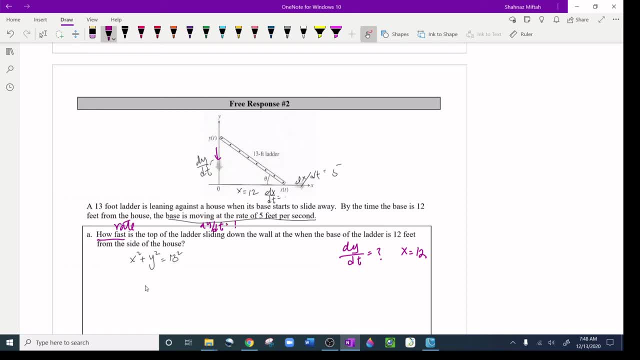 square plus y square equal 13. square 13 is constant, so let's take a derivative of this. if I take a derivative of that, it's 2x DX DT plus 2y dy DT equals 0. now X is given. I don't have a y and dy DT I'm looking for, so how would I get that y? I'm 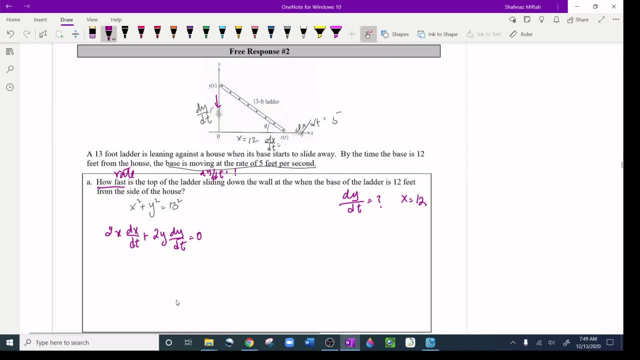 going to use a Pythagorean theorem again to get that, to get that y. so how would I get that? let's see x square, which is 12 square, y square is missing and that's 13 square, so that's 144 plus y square, equal 13 square is 116.4. 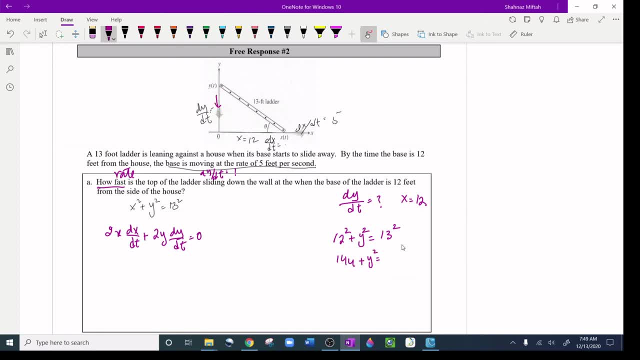 169. so far I remember 13 square is going to give me 169. 169 subtract 144, it's going to give me 25. so y square is equal 25. now square root it, so y is equal 5. so this is what I got. 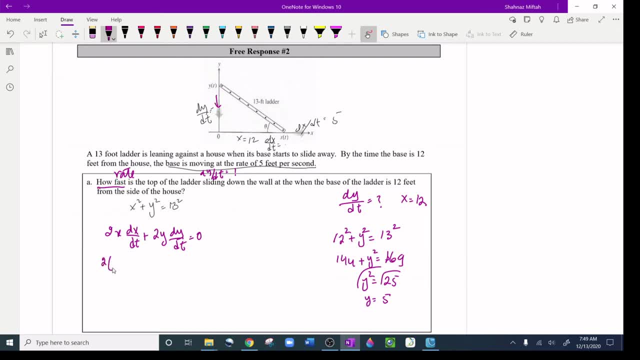 now let's plug in everything. now we have everything. two times X is 12, DX DT is five. two times five and dy DT- oh, that's a plus sign, sorry, dy DT- is going to stay equals zero. um, what can I do? 12 times five, 24 times five is going to give me 120. 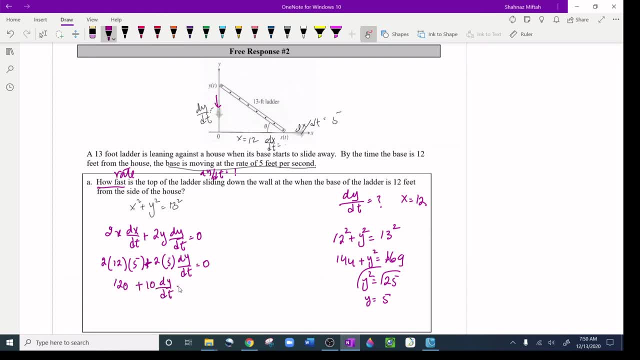 plus 10 dy DT equals zero. now move the 120 to the other side. 0 and 120 are like terms. 10 dy DT equal negative 120 and divide by 10.. so that's negative 120 divided by 10 is going to give me 12.. so I have dy DT equal negative 12 and 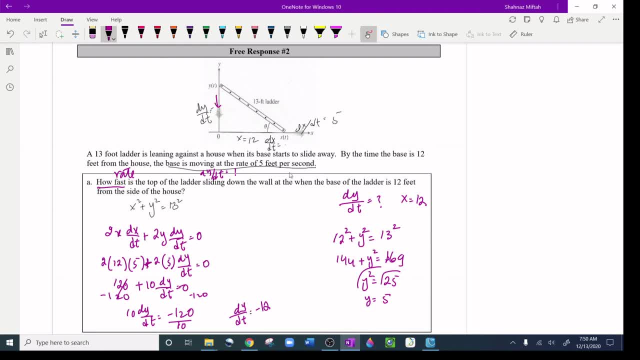 since this is dy DT, my units are around feet per second. my units are around feet per second. part is going to come because of the um rate. that's a rate, so it's a negative 12 feet per second. that's the answer. this part is uh has three points. one point is uh. using this formula: 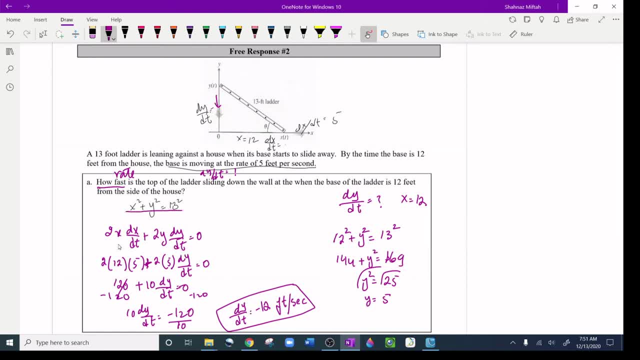 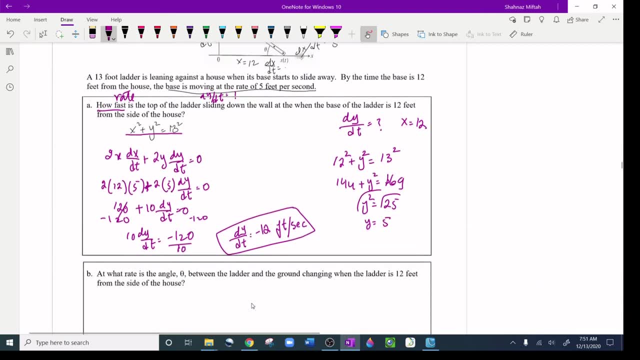 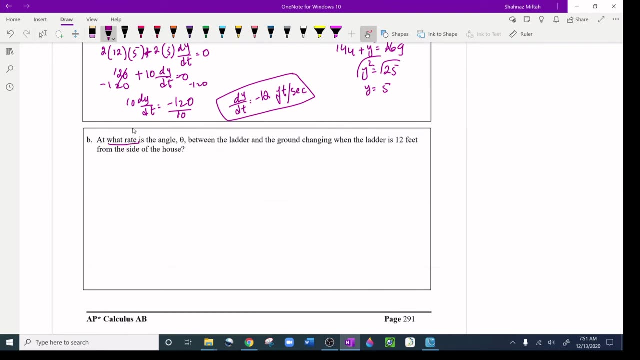 that you figure it out. it's supposed to be pythagorean and, um, you took a derivative. that's second point and the answer is the third point. so that's part a. here is a part b. at what rate is the angle theta? what rate? again, d something dt is there is the angle theta. so d theta, dt. 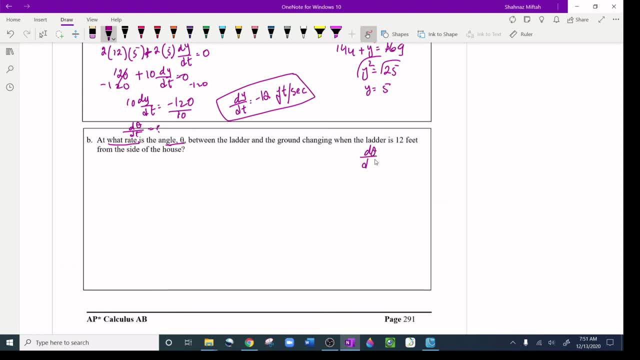 is missing. uh, i'm looking for d theta, dt question mark between the ladder and the ground changing when the ladder is 12 feet from the side of the house. so this is again. the x is going to be um, the x is going to be again, uh, 12. 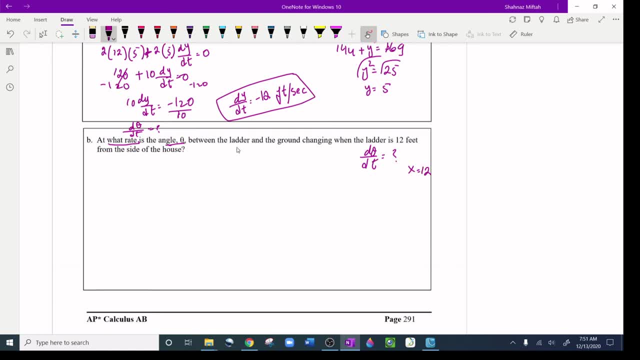 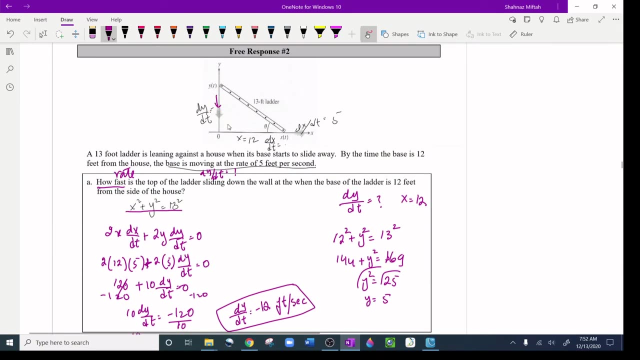 okay, so now i'm using a sohcahtoa because they are talking about theta angle sohcahtoa, so let's see which one would work for us. so let me check that. okay, which one? can i do opposite? uh, if i do sine, so sine is going to be 12 feet from the side of the house, so 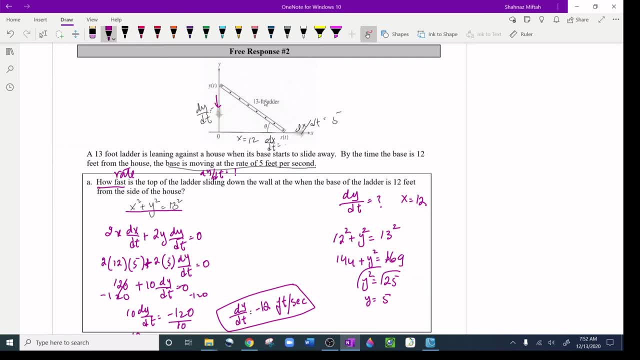 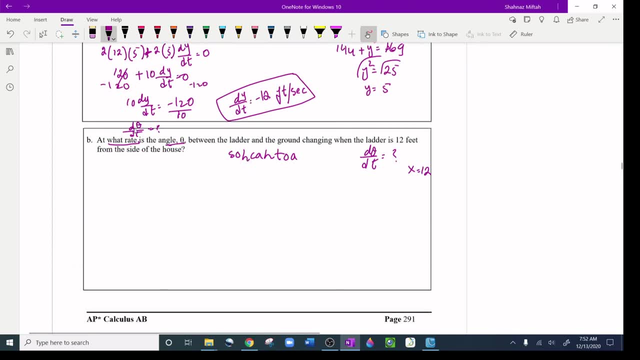 sine is going to go opposite over hypotenuse. hypotenuse is 13, opposite is y. since the question is talking d theta dt, all three of them would work because i'm talking about d theta dt. so if i'm doing sine, theta equal, opposite was y and hypotenuse was 13. so, um, let's take a derivative of this. 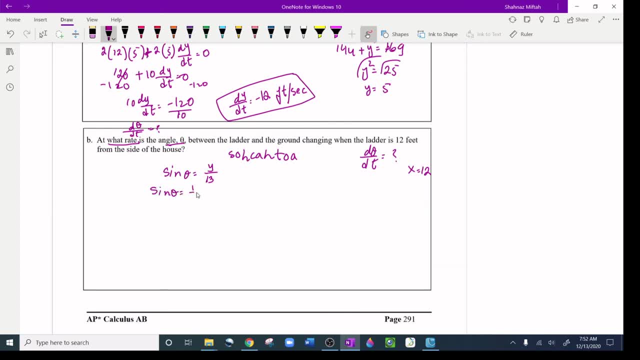 rewrite this first, because 13 is in the bottom. i can write like 113 y so cosine theta d, theta dt. 1 over 13 and dy dt. now d theta dt. i'm looking for. dy dt is given, which is negative 12 we already got. 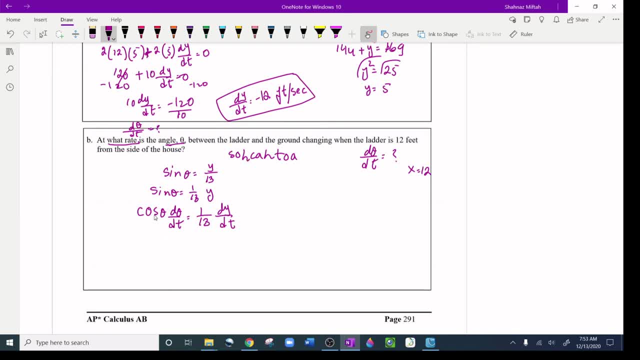 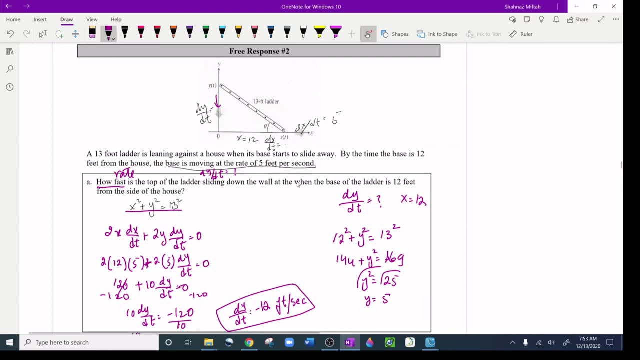 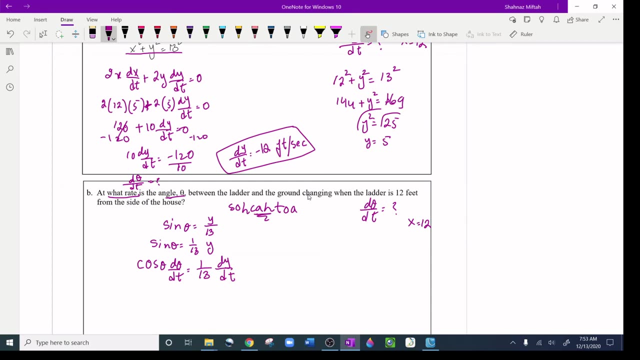 this in part a. so now let's do: what about cosine theta? what is cosine? cosine means adjacent in hypotenuse. so which one is adjacent? 12 over 13.. that's, 12 over 13 is my adjacent, so 12 over 13. i'm going to write there: 12 over 13. d, theta, dt i'm looking for. 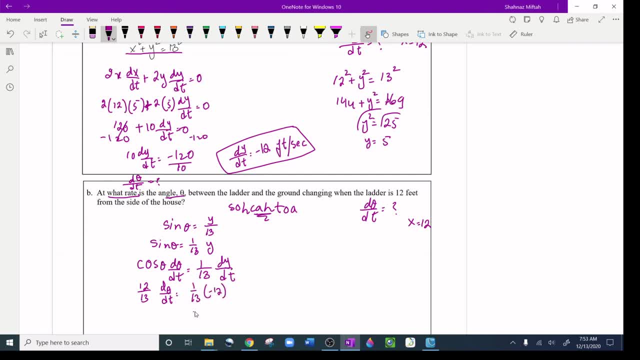 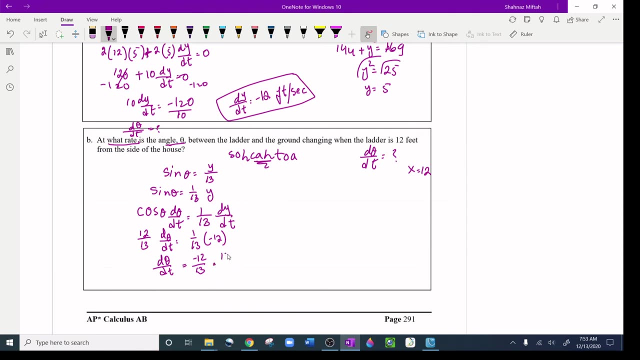 1 over 13, times negative 12.. so this is negative. 12 over 13, equal d theta dt and 12 over 13. this 12 over 13. i'm going to multiply both sides, the reciprocal, so it's going to be 13 over 12.. cancel, cancel, cancel, cancel. so d theta dt is equal negative 1, and since this is 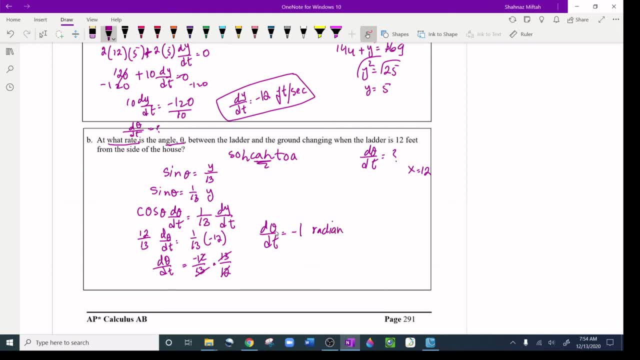 an angle, it's supposed to be radians and since it's a derivative, it's going to be per. and uh, what am i using? radians per second. so this part of the question, like this part b, has three- um what is it called? three points: one point by using correctly the sine, or cosine, or 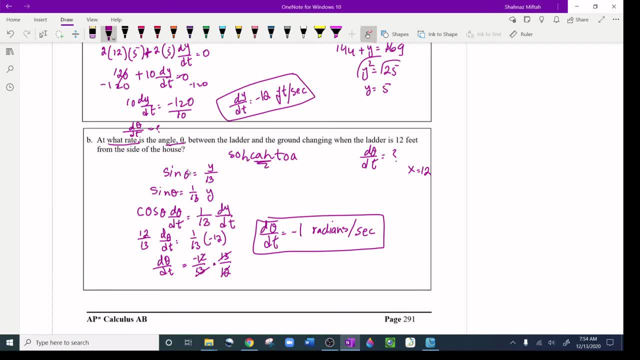 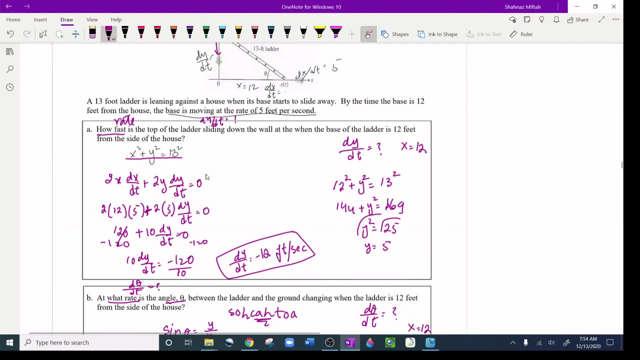 tangent, whatever you want to use, whichever works. so, uh, that's what it is. and uh, i used sine because you know dy dt was given, so i can easily do the y's of that. if you do the x's, then it's not given here dx dt is not there. our dx dt is five. you can do x, two, okay. 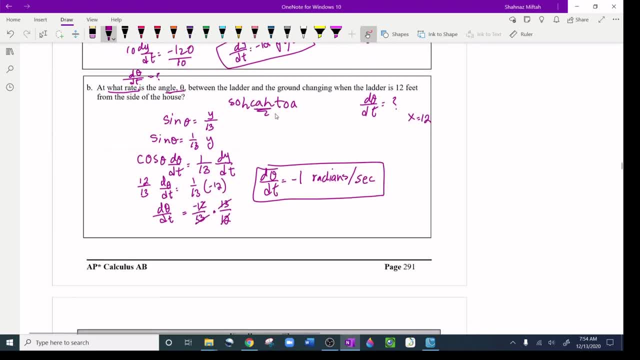 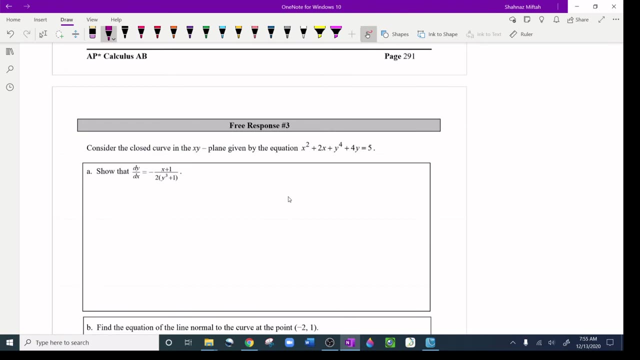 okay, this is what i got. so one point is for picking the right formula of the trig, second is derivative and third is answer. so these are two questions. now free response. part three: in this case, consider the closed curve in the x- y plane given by the equation this: 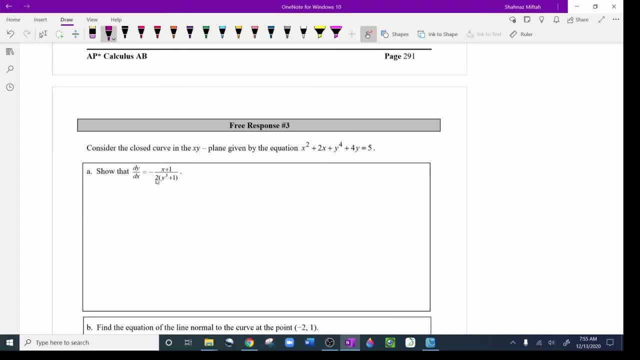 show that d by dx is equal negative x plus one. show that, which means you're taking a derivative of this, and get to this answer. this is the answer, that's. this is the derivative of this question, so we have to just show them the steps. so x square plus two, x plus y, fourth plus four, y equal five. 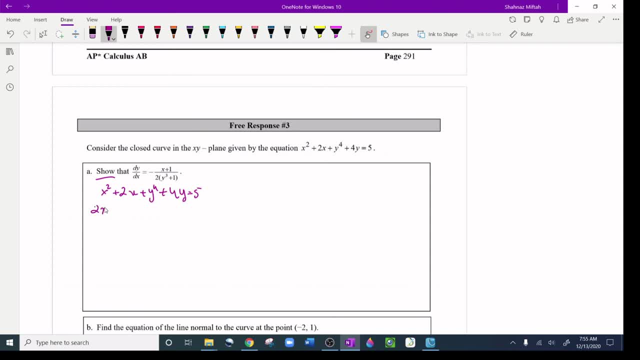 now take a derivative and see if we're getting this. so two x, and since this is implicit, i'm going to have a dx, dy over dx. since i'm taking a derivative of x, that's going to be dx, dx. we don't write that derivative of two is again that four y. 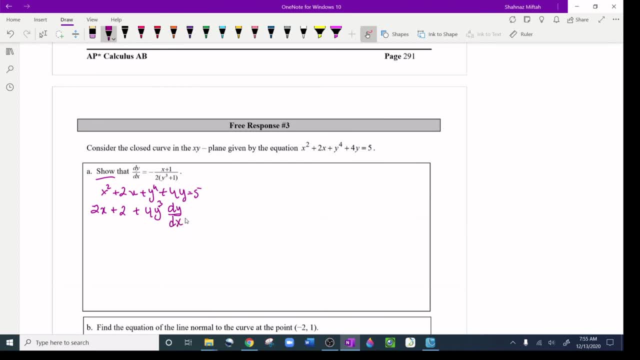 cube and this is going to go. dy dx plus four dy dx equals zero. keep the dy dx is on one side, the rest of the stuff to the other side. four y cube dy dx plus four dy dx equal. negative two x and negative two this one. i moved it to the other side of equal. now dy dx is a common factor. 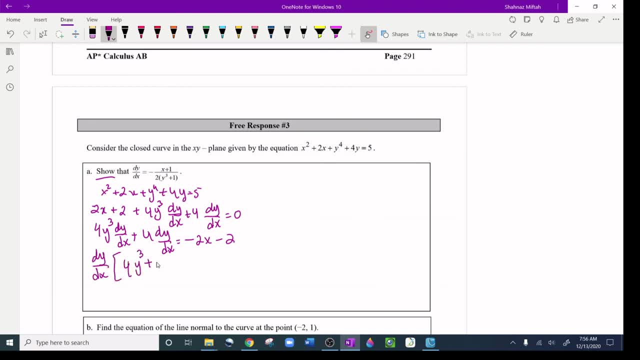 left with four y cube plus uh, four equal negative. two x minus two divide both sides: four y cube plus four. four y cube plus four. now can i do anything else here to simplify this? uh, yes, i can. i can do common factor, remember four, five. i think we have properties of operations that we consider after the derivative lcd common factor. 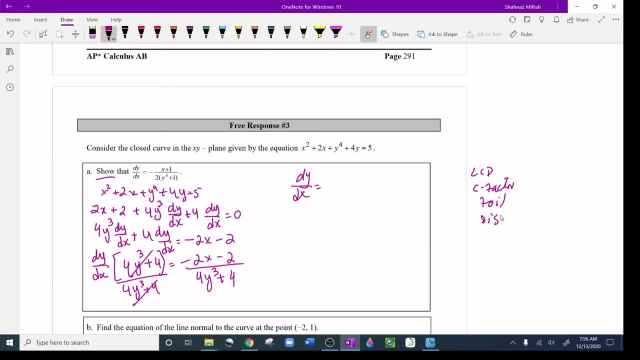 common factor, because we are left with x and i am left with plus two exponent properties. now if we want to distribute this common factor, this is one of the common factor function. also, i'll add the random variables of each of these. it'll be a common factor coordinate. so let's say i have two stuffs here. this is going to be one of different operations. so now let's deff the foil, distribute to us the common factor. so now i am left with sequential properties: 1, 2, 3, 4, 5 and, uh yeah, five different operations that always remember if you get stuck after the derivative. so now um 2 is the common factor. so, ah, yeah, so i going do the two common factor, which will give me negative two common factors. so i'm left with x and i am left with plus three. So now 2 is the common factor. so I am going to do the two common factor, which will give me negative two common factors. so in particular, i have one that my good foreign°. is that all the common factor? so i am left with that x and I'm left. 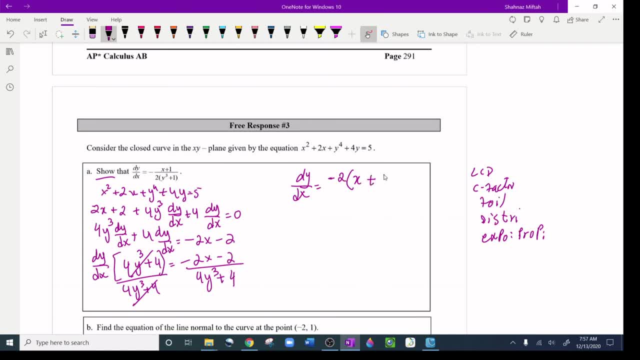 common factor. so i'm left with x and i am left with plus one. in the bottom two is a common factor which will give me two y cube plus two. this two to cancel out, i'm left with negative x plus one over two y cube plus two, and that's exactly what i have up there. they also getting. 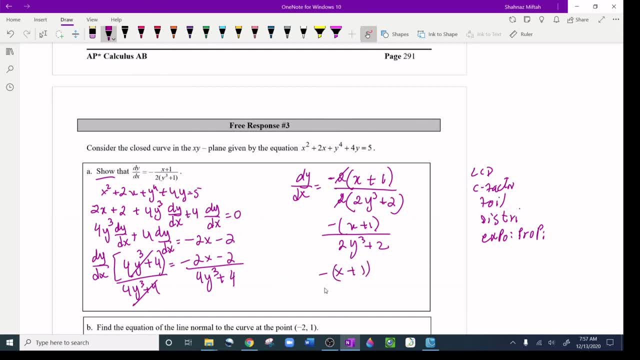 the again, the two, um uh, common factor again. so i got y cube plus one, y cube plus one, and that's exactly what i have here. so that's my answer for d, y, d, x. there you go, and this part has two uh points: one point taking a correct derivative and the second point getting the answer. 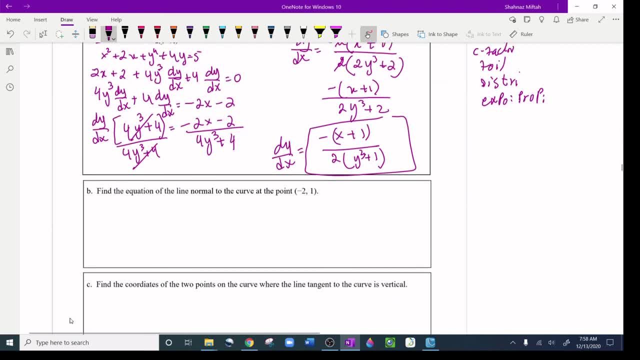 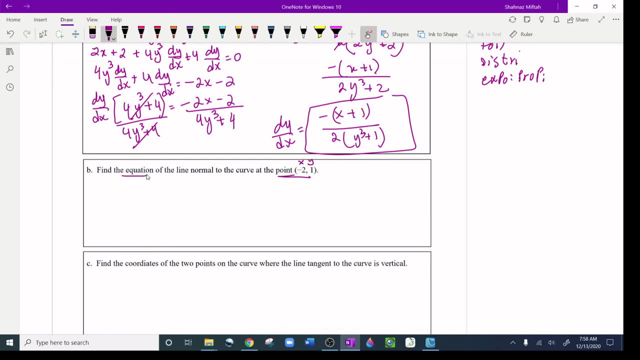 okay, part b of this question. find the equation of the line normal to the curvate point. point means: this is x. that's a y equation means y minus y, 1, equal m, x minus x, 1.. so that's an equation. now, um, let's figure it out everything. a normal line. 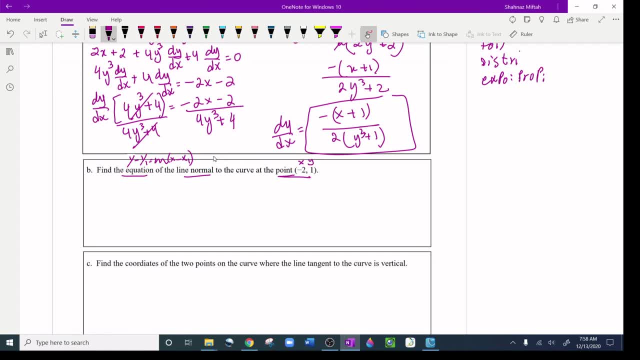 remember: normal and tangent goes reciprocal and opposite. reciprocal and opposite like they go back and forth, the normal and tangent line. so equation is: y minus y, 1, equal m, x minus x 1.. the points are already there. all i need a slope. so what is the slope of the equation? we got the slope right here. all i have to do is plug in. 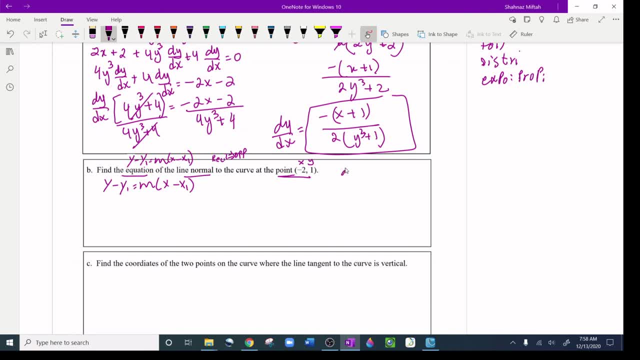 negative 2 and 1 here to get that slope. so i have a slope dy dx. you know, dy dx is a slow, like a derivative: x plus 1 over 2 y cube plus 1. i'm using this and i'm plugging in the values and 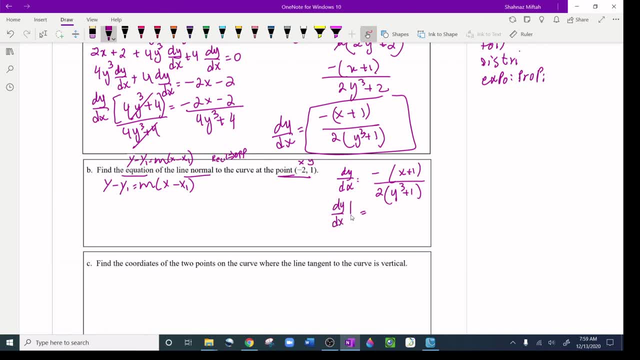 this is anotherставляve world. uh, the values here here- this is another thing you guys should see- draw a line like a vertical line and right at the bottom negative 2, 1, which means I'm plugging in now these values for the derivative, so I got negative. 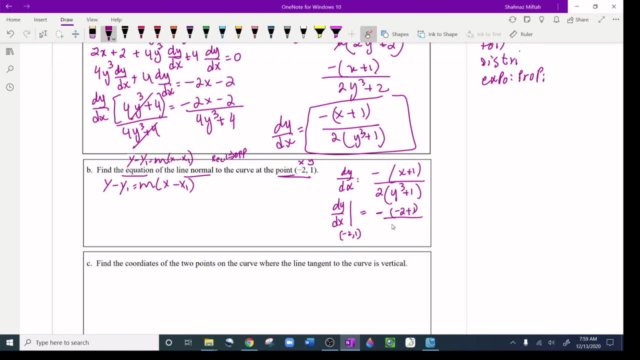 negative: 2 plus 1. the bottom 2 y is 1 plus 1, y cube plus 1, so it's technically gonna give me 1. 4th, like: hold on negative times. negative is positive and it's gonna get negative 1. let's do it: negative 1 in the bottom. I got 2 and 2. 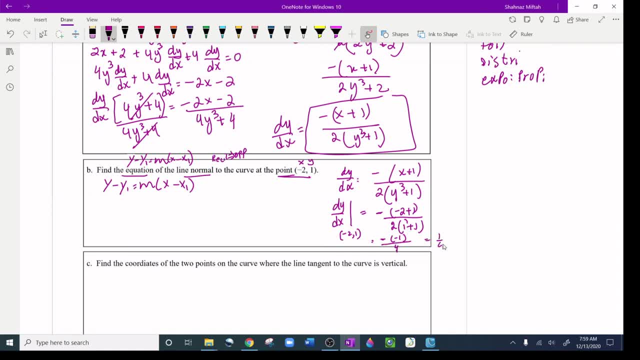 is 4, or negative, negative is positive. so I got positive 1, 4. so the slope is positive 1: 4. so y minus y, 1 is 1. slope is positive: 1, 4. X minus negative, 2, which turns positive. so that's my equation of the this: 1. 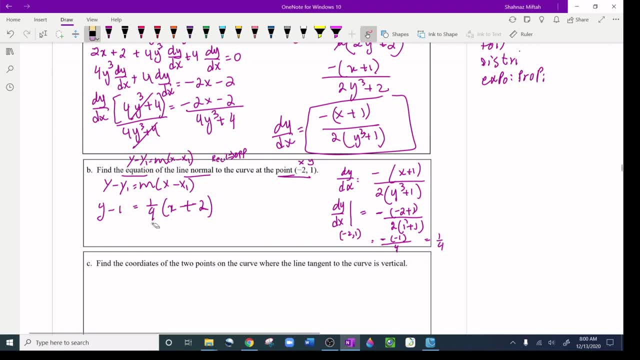 fourth is the tangent slope. okay, I should not put this. my equation is for normal line, so I: this is the tangent slope that we got. this is tangent slope. we know that because that's a derivative. that's a tangent slope. for the normal slope it's gonna go reciprocal in opposite, which means it's gonna go. 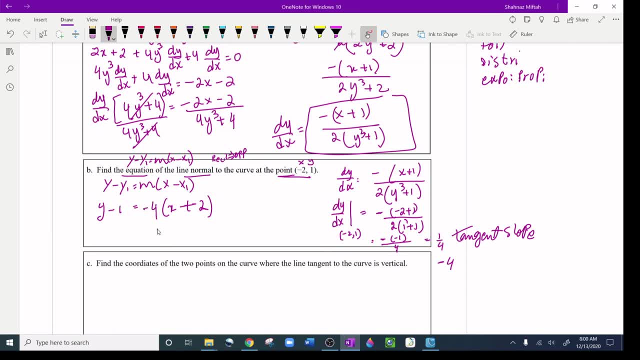 negative 4. so negative 4 and this is done. this is the normal line. normal line slope, reciprocal and opposite, and this is what my equation goes. this question has two points: one for the answer, like the whole equation, and again next, at one point, is finding this value like negative 4. you get the tangent whole steps 1, 4 and then 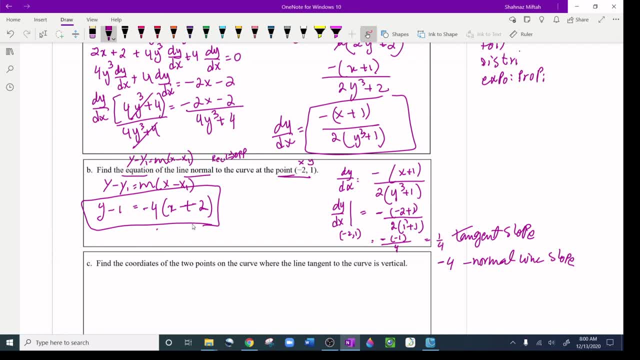 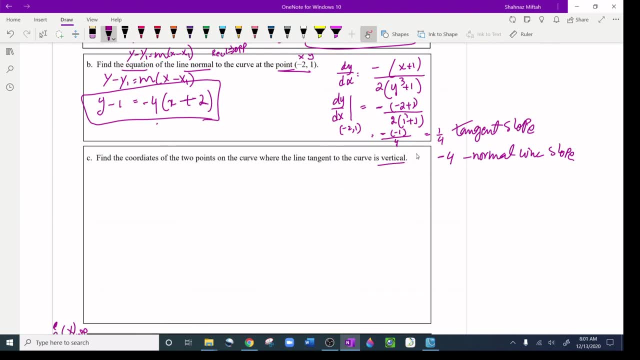 you get this. this whole thing is one point. this is another point. part c: find the coordinates of two points on the curve where the line tangent to the curve is vertical. vertical means when it's undefined. so undefined means we should have one over zero, something like that. tangent means derivative. two points like x and y's coordinates. 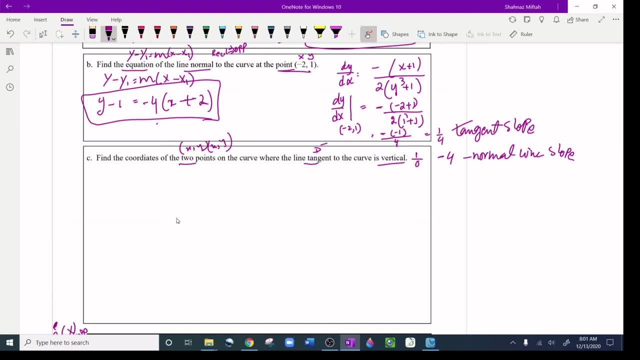 like this one point and that's a two point. so now what can we do? we have the derivative and we're going to make it equal this. so derivative is negative: x plus one over two y cube plus one, equal one over zero or undefined. so you cross, multiply, i am getting two y cube plus one. 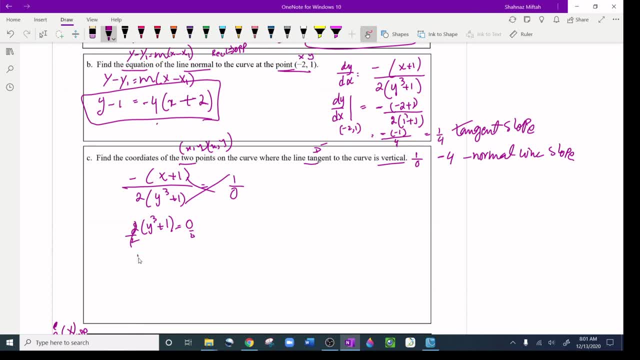 equals zero. you divide two, both sides, and i am getting y cube plus one equals zero. so this is what i got: y cube equal negative one. so i got y equal negative one. so i got negative one, which is the y value. now, since they are asking two, 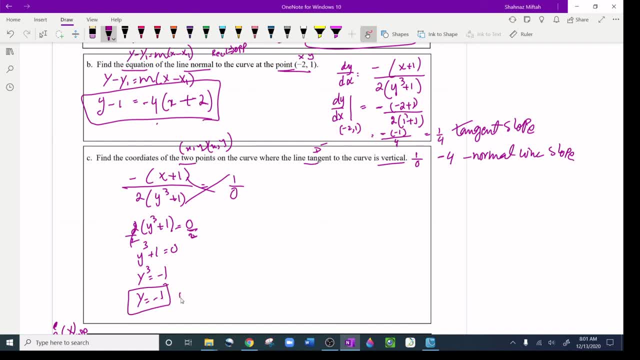 coordinates. so it means i'm plugging in this y in the original, in the original equation, plug in. so what is my original equation? it's 2x plus 2y. i think that's what it was, if i'm not mistaken. i have to check back. 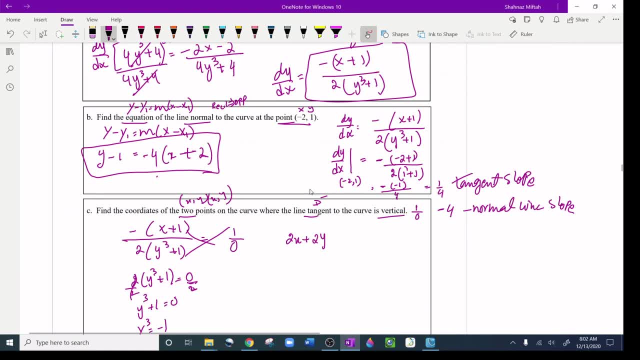 x square plus 2x. okay, that's the derivative i'm writing, so let's erase that. i got x square plus 2y, 2x plus y4, 2x plus y4 plus 4y equal 5, plus 4y equal 5. so always you. i told you guys before when: 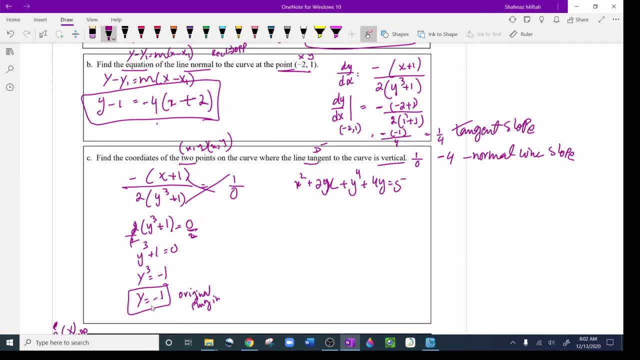 always you're missing x or y and or any one of them. you've already figured it out. like you, either x or y, you figure it out, and missing another one, plug it in in the original. so my x square plus 2x plus negative 1 to the power, 4 plus 4 negative 1 equal 5. it's going to give me. 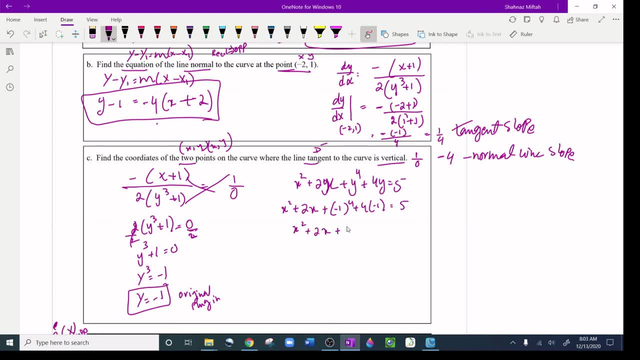 x square plus 2x plus 1 and negative 4 equal 5. this is going to give me negative 3 equal 5 and i got x square plus 2x. i got all of that. now, um what else i can do here? i move the 5 and make. 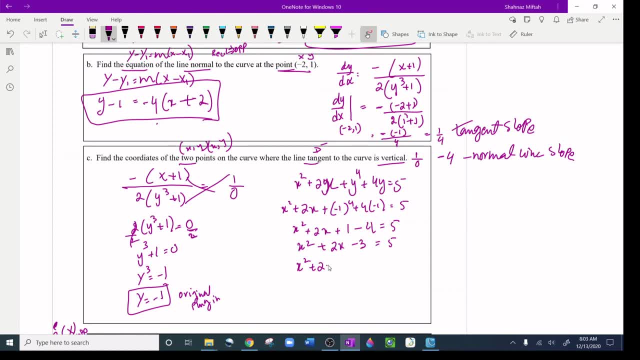 a quadratic. since it's already a quadratic, we can factor out: negative 3 minus 5 equals 0, 5, 6, 7, 8. negative 8 equals 0 and 2x plus x square. now, what are the factors here? factors are um x plus 4 and x minus 2, because 4 times 2 is 8 and 4 subtract 2 is 2, so 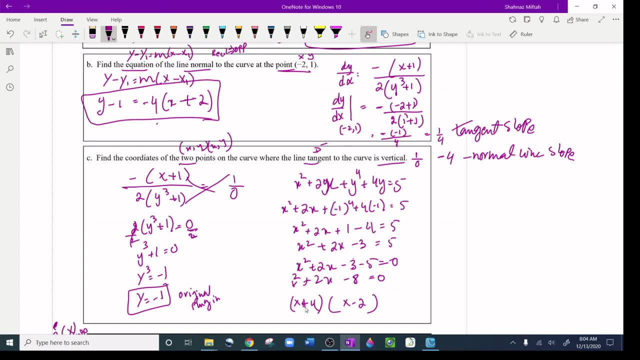 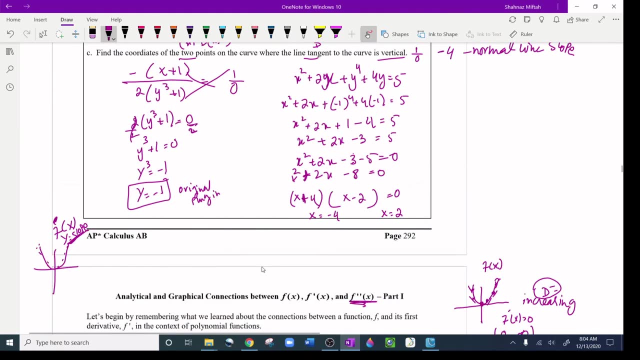 the positive sign supposed to stay here because it's a bigger number. so my equals 0. now what are my x's? i have got x equal negative 4 and i got x equal positive 2. so these are my uh, two points, and i'm gonna write down these two points like really like an answer.